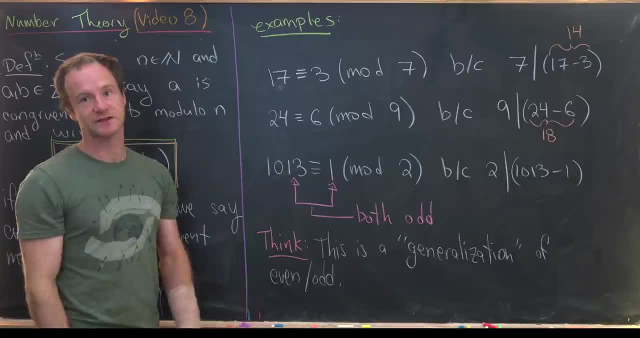 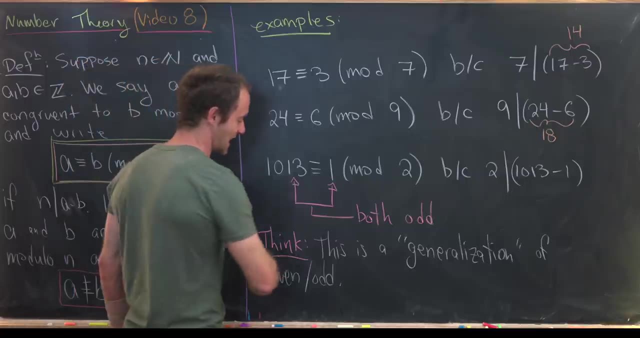 2, because 2 divides well 1,012,, which is the difference of those two numbers. And how you want to think about this is that you want to think about the difference between the two numbers. So you want to think about this is that this notion of congruence, modulo n, is a generalization of 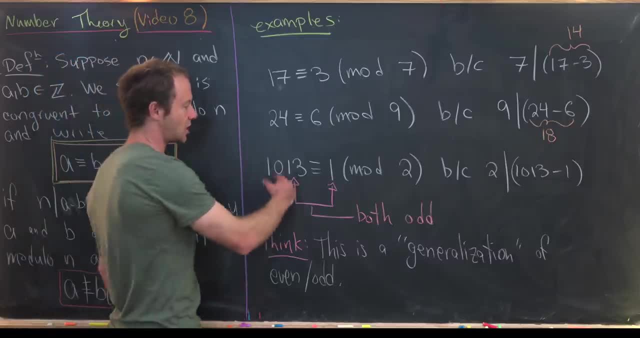 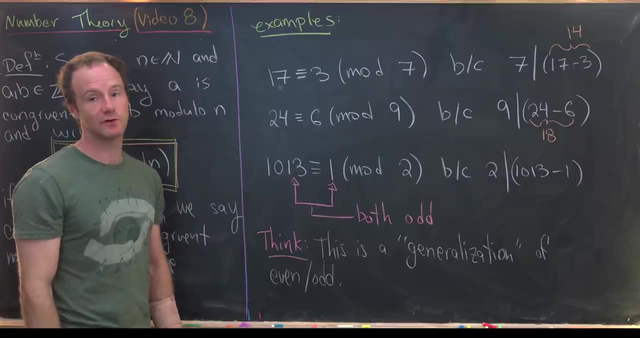 even and odd numbers. So notice: all odd numbers will be congruent to 1 modulo 2.. And all even numbers will be congruent to 0 modulo 2.. So there are two choices when we're talking about congruence modulo 2.. But there are n choices when we talk about congruence modulo n. So instead of just 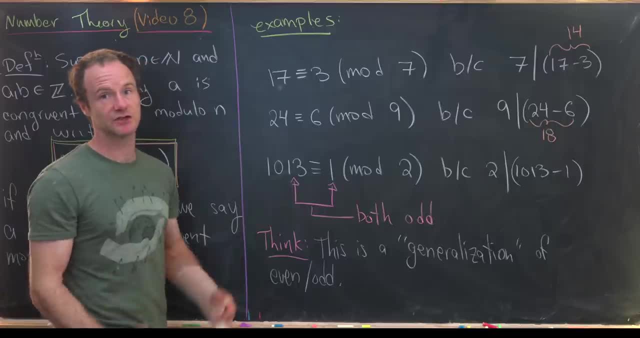 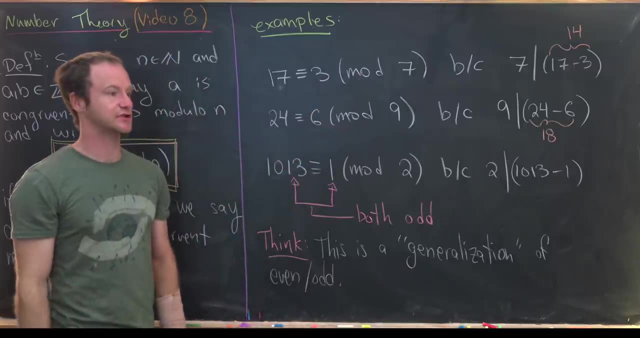 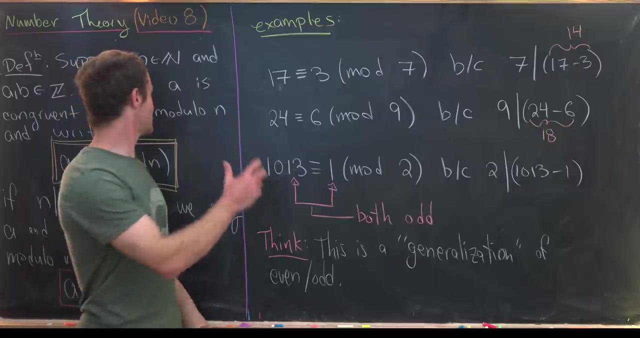 having two choices, even and odd. we have n choices. So like for example up here when we're working modulo 7, things can be congruent to 0,, 1,, 2,, 3,, 4,, 5, or 6 mod 7.. Okay, so let's maybe get rid of these. 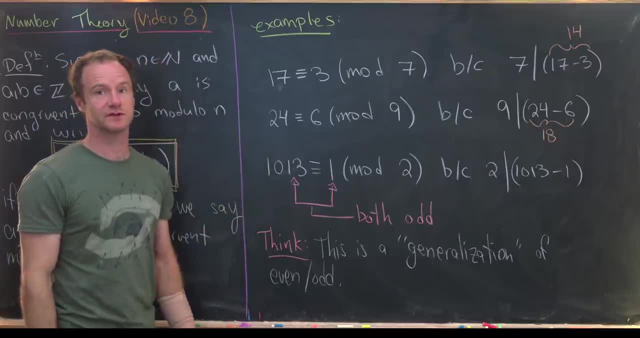 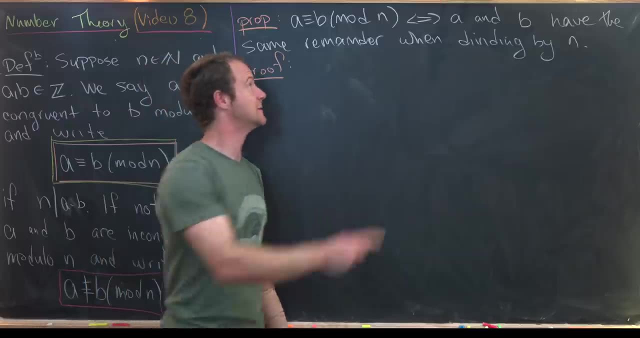 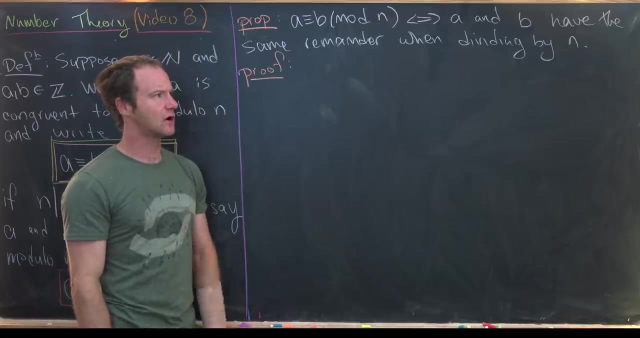 examples And we'll start proving some standard results. Okay, so our first claim that we will prove is that a is congruent to b modulo n, if, and only if, a and b have the same number of numbers. So we can divide them by n. So, let's recall, using the division algorithm, we can always divide one. 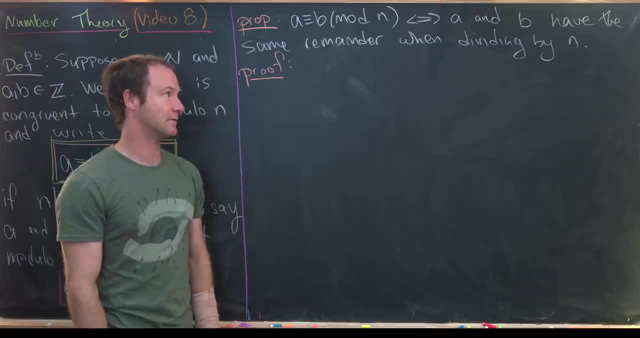 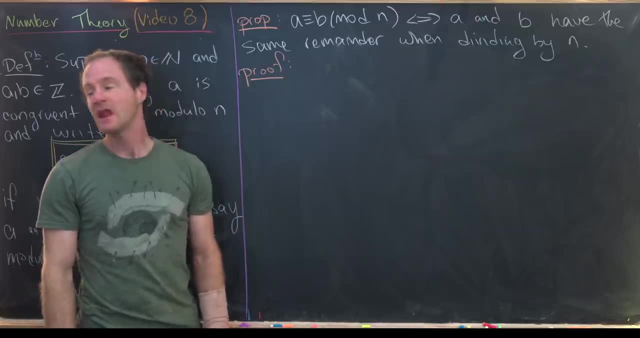 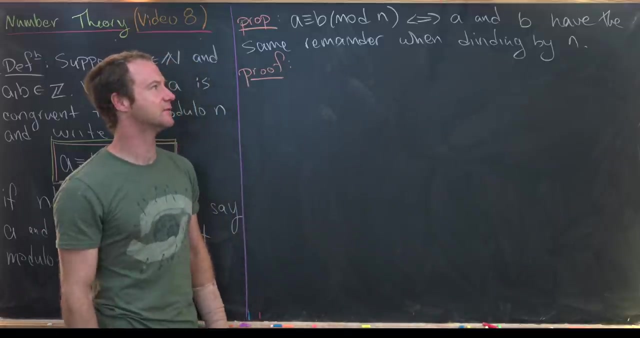 integer by another integer and we pick up a quotient and a remainder. What this is saying is that this congruence modulo n only depends on the remainder, And while this over here is the precise definition of congruence modulo n, it's generally a little bit easier to think about. 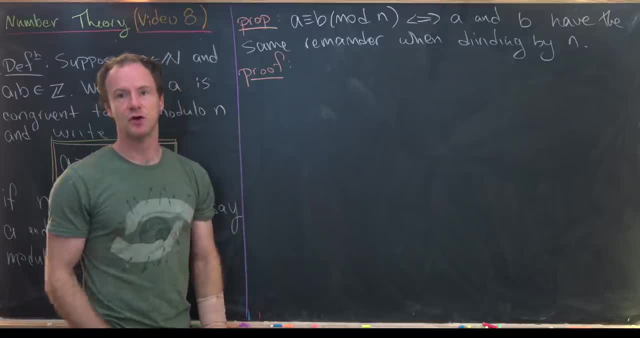 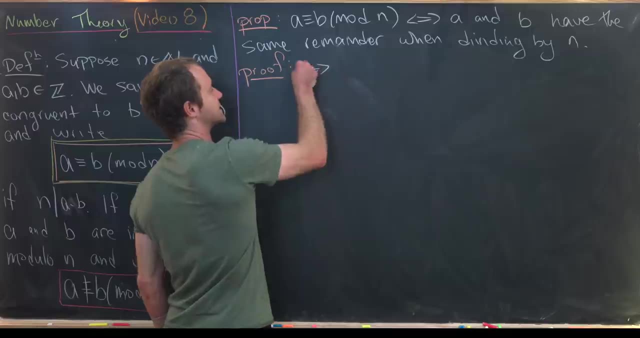 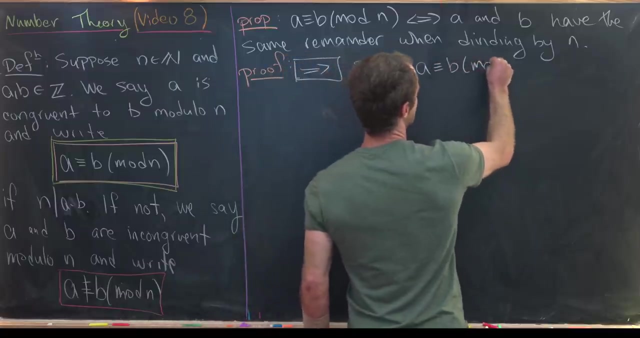 congruence modulo n via this proposition. So let's say that b is congruent to b modulo n and b is congruent to b modulo n. Okay, so let's maybe go ahead and prove that. So we'll prove this forward direction first. So let's suppose that a is congruent to b modulo n. So by the definition, 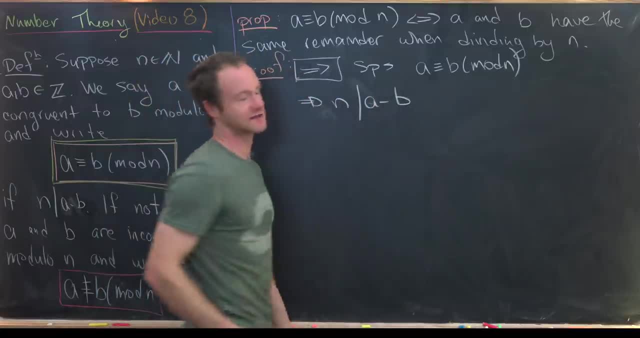 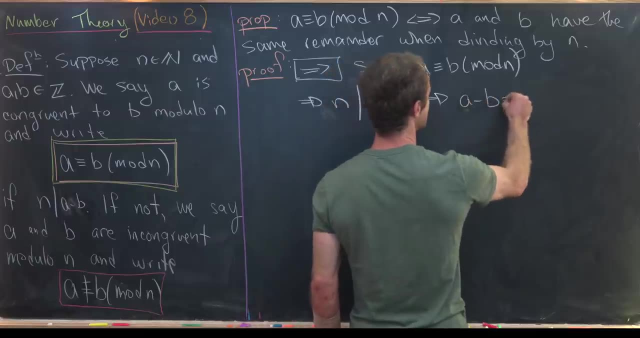 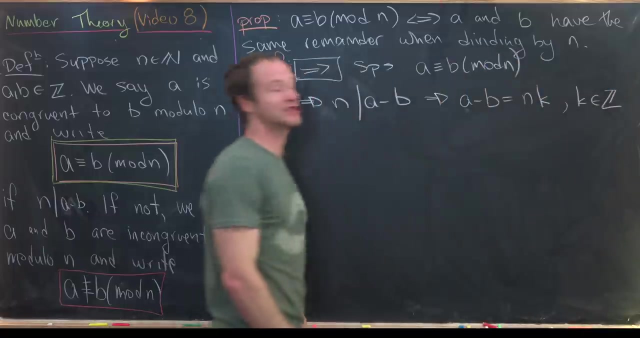 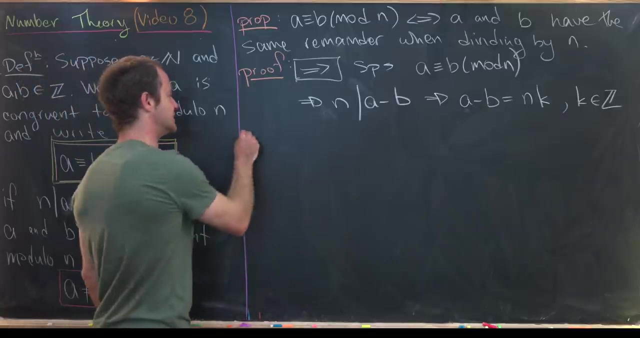 that means that n divides a minus b. Okay, but that tells us that a minus b can be written as n times k for some integer k. That's just the definition of divisibility, Okay. so now that we've got that sorted out, let's maybe go ahead and use the division algorithm. 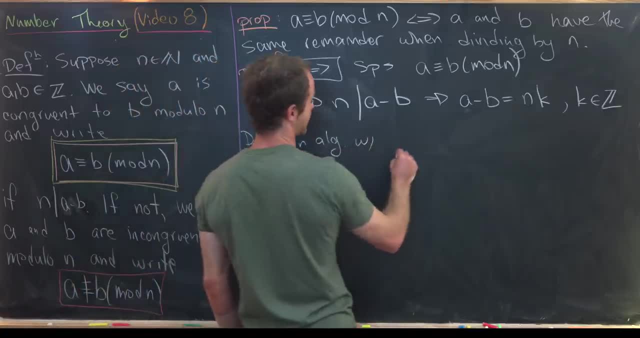 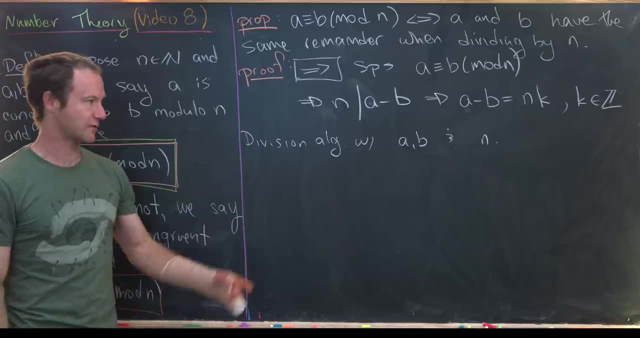 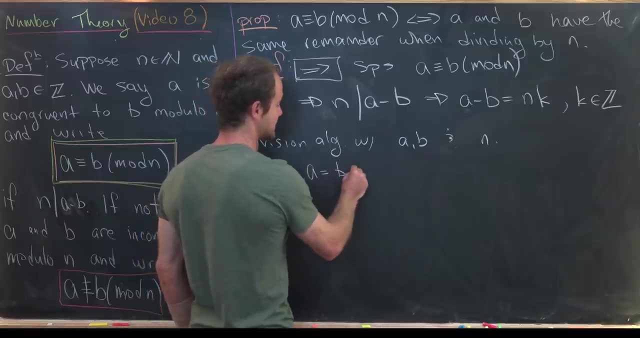 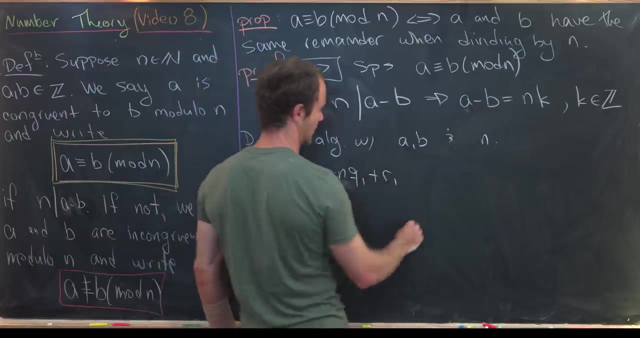 with a, b and n. So we're going to divide a by n- have the quotient and remainder- and b by n- have the quotient and remainder. So that means we can write a as b times q1, as n times q1 plus r1.. And notice that r1 is going to lie between 0 and n. It's allowed. 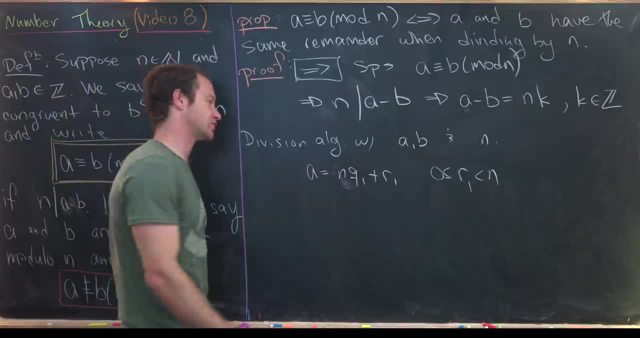 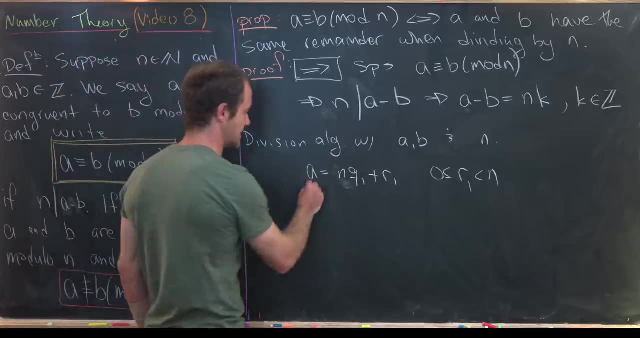 to be 0,, but it's not allowed to be n. So just to reiterate, we, divided a by n, had a quotient of q1 and a remainder of r1.. We'll do the same thing for b. So we have: b is equal to n times q2. 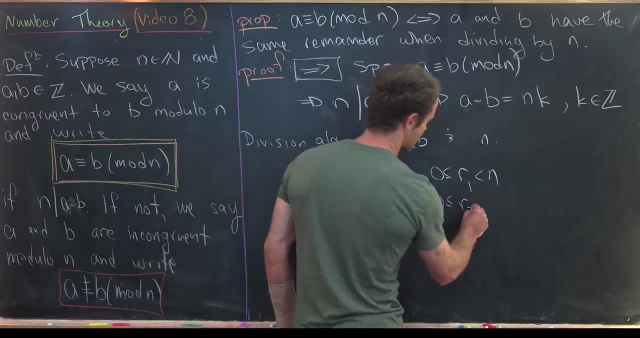 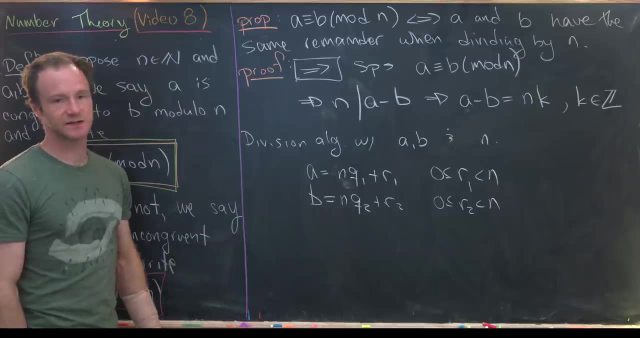 plus r2.. And likewise we have: r2 is between 0 and n, including 0, but not including n. Okay, nice, So now where can we go from there? Well, we know this thing up here, that a minus b. 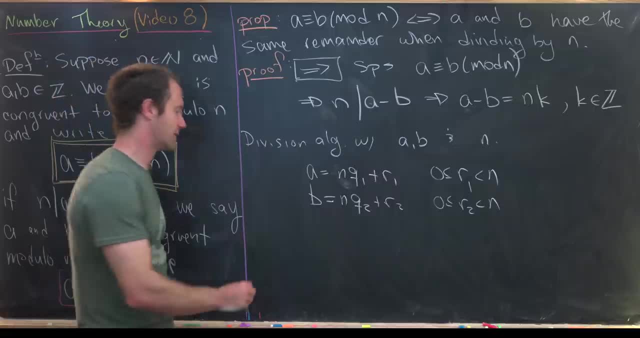 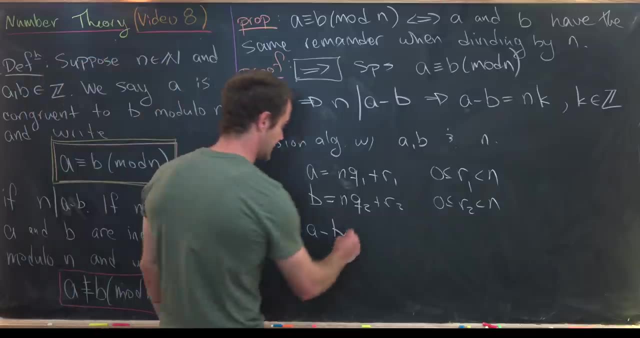 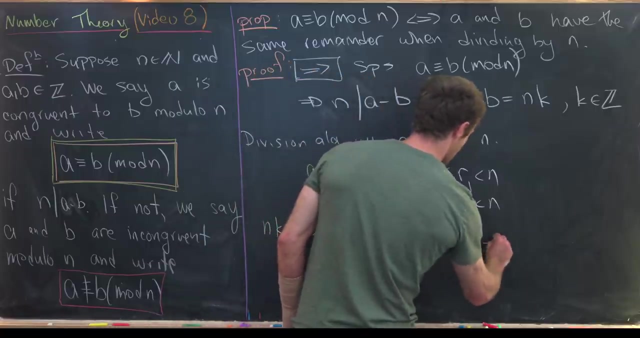 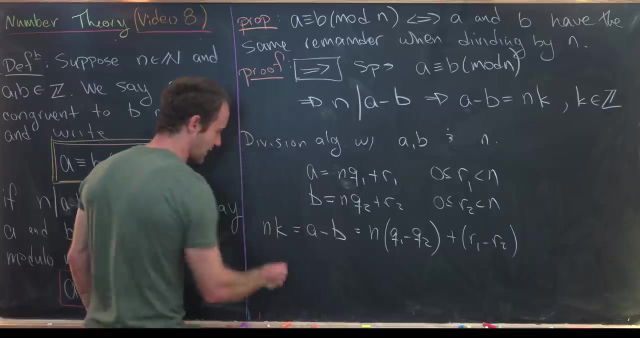 is equal to nk, So maybe we want to look at that. So we've got n times k is equal to a minus b, But that's the same thing as n times q1 minus q2, plus r1 minus r2.. Okay, But notice that this guy right here is a multiple of n. 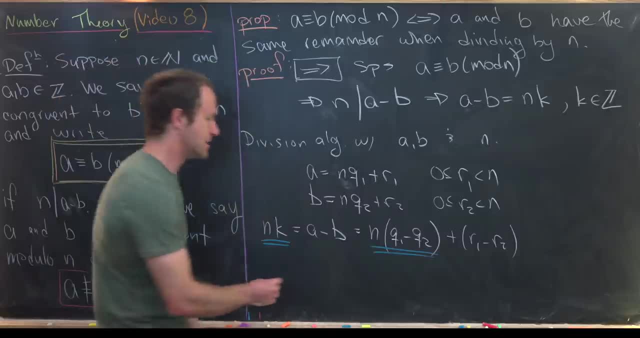 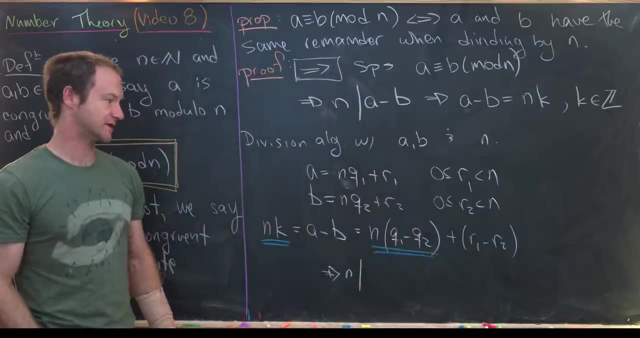 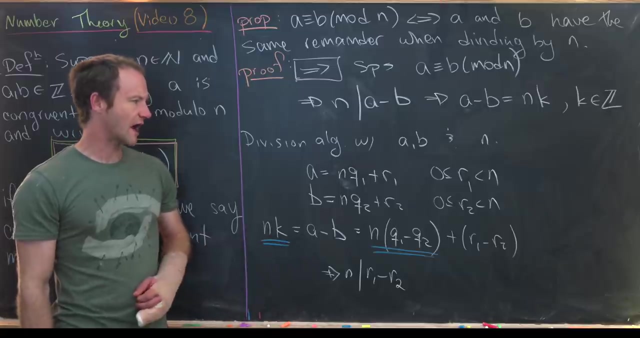 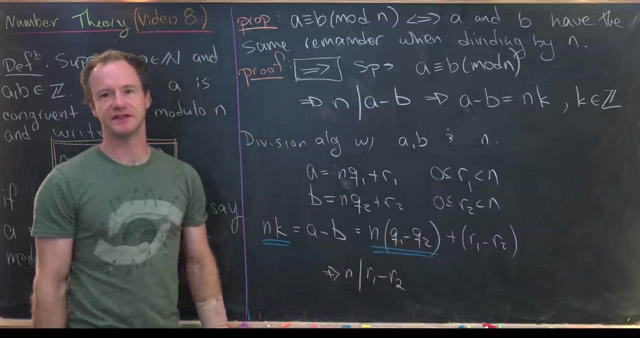 This guy right here is a multiple of n, But that tells us that n divides whatever's left over, which is the difference of these remainders. So n divides r1 minus r2.. But now let's look at the range of r1 and r2.. So r1 is between 0 and n and r2 is between 0 and n. 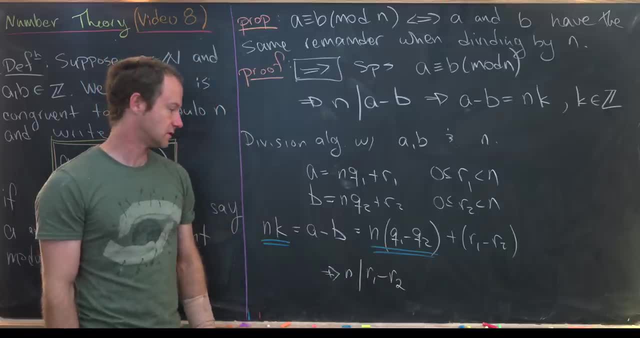 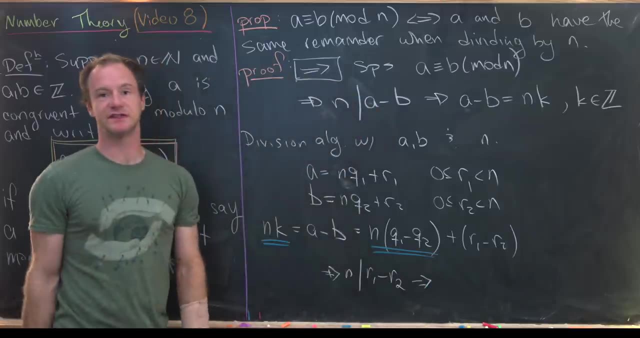 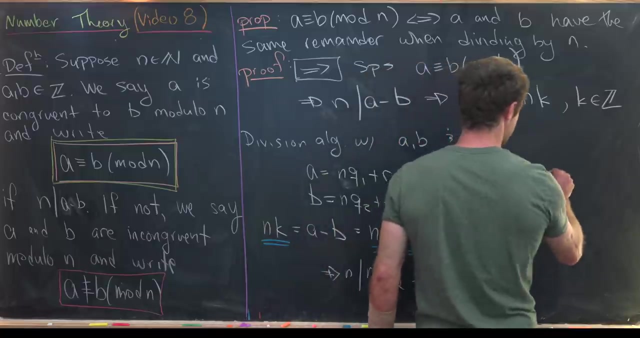 But this kind of divisibility is impossible unless r1 is equal to r2. In other words, unless this is equal to 0. And why is that? Well, that's because this over here implies that r1 minus r2 is equal to 0. So r1 minus r2 is equal to 0. So r1 minus r2 is equal to 0. And so? 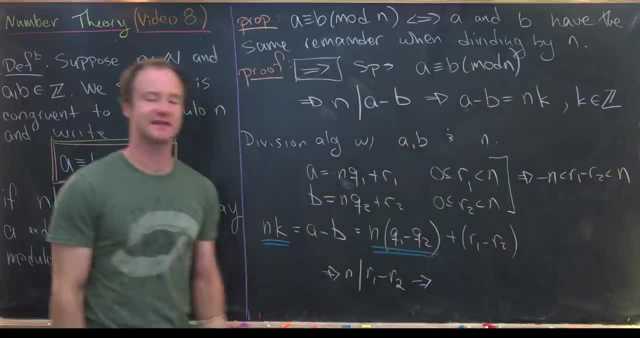 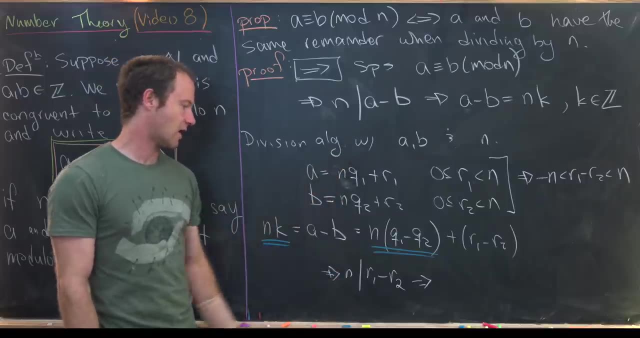 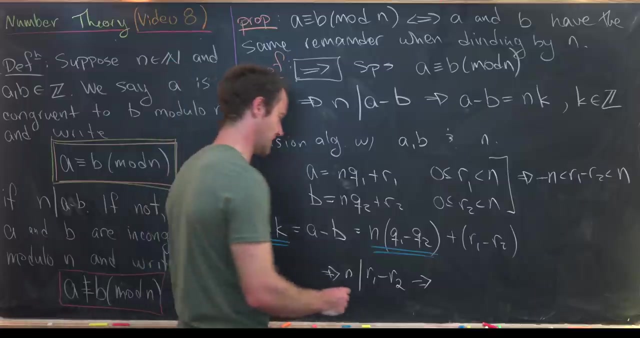 r2 is going to be strictly between minus n and n. So since r1 and r2 are between minus n and n, and r1 minus r2 is divisible by n, well, that means that it has to be the zeroth multiple of n. 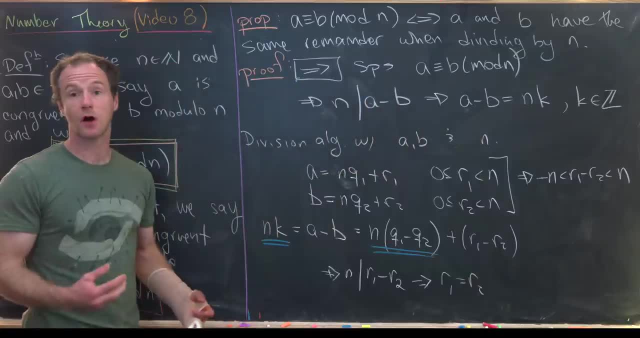 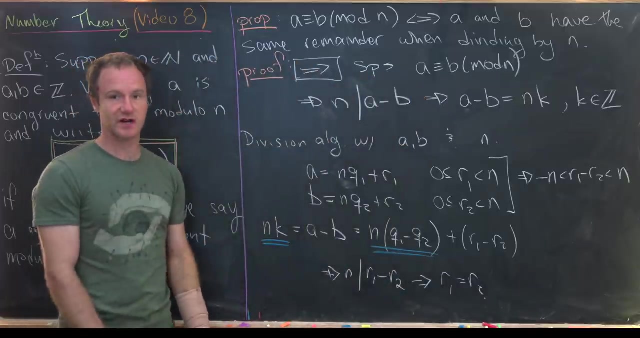 In other words, r1 equals r2, because r1 minus r2 is equal to zero. Okay, but look, that's what we have on this other side of our implication. a and b have the same remainder when dividing by n. So we finished this first direction. Now let's go ahead and look at the reverse direction. So we 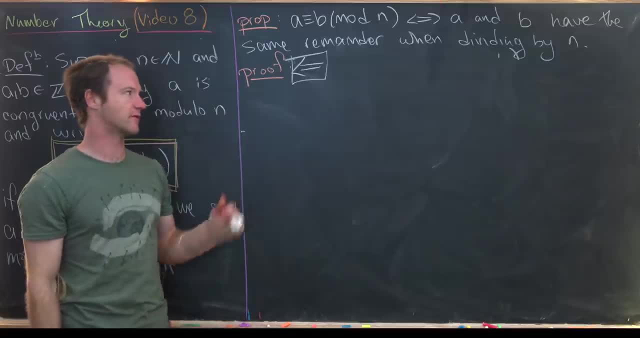 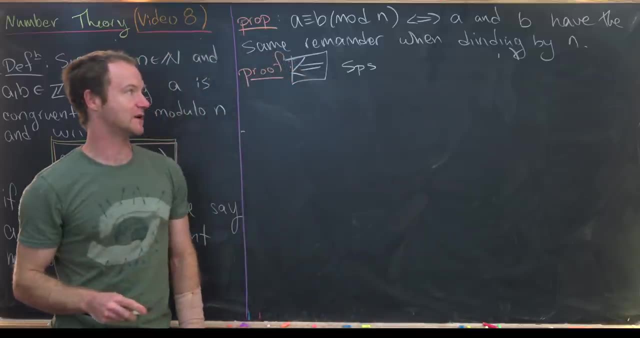 just finished proving the forward direction, and now we're ready to prove the reverse direction. So what we'll do is suppose that a and b have the same remainder when dividing by n. In other words, we can write a as n times q1,. 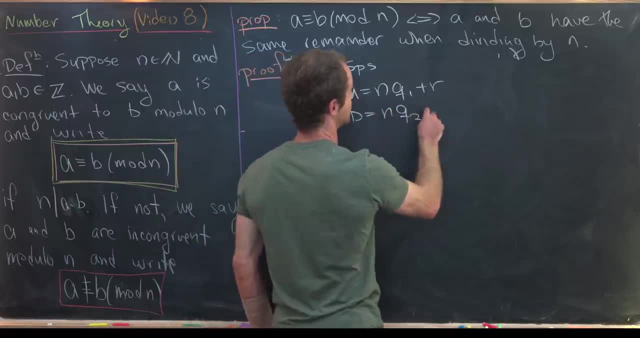 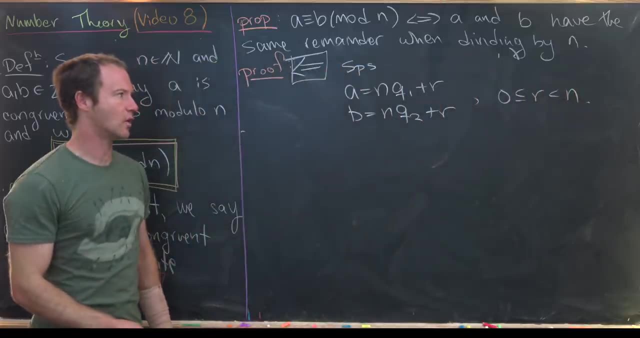 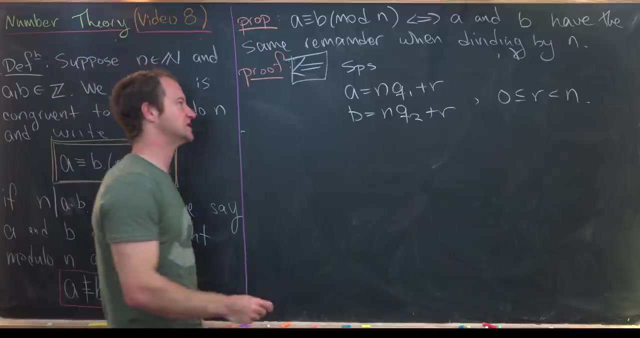 plus r and b as n times q2, plus r, And here r is between zero and n. Notice I didn't need r1 and r2 here, because our assumption is that we have the same remainder. But now we're pretty much good to. 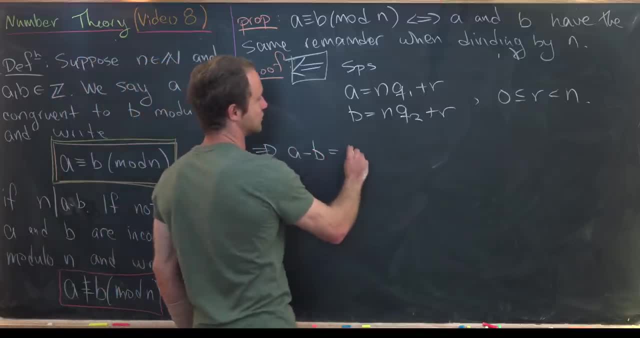 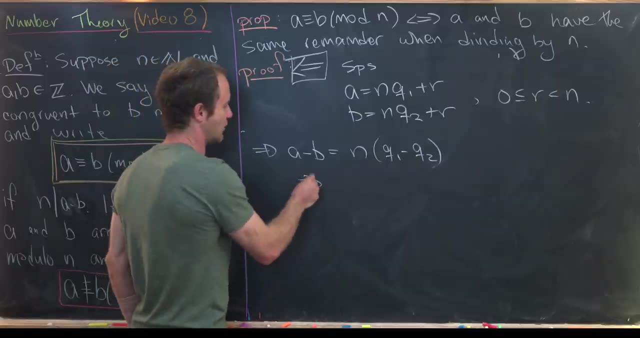 go, because we have that a minus b is equal to n times q1 minus q2, because the r's cancel. But that's exactly what we need for n to divide by n. So we have a minus b is equal to n times q1,. 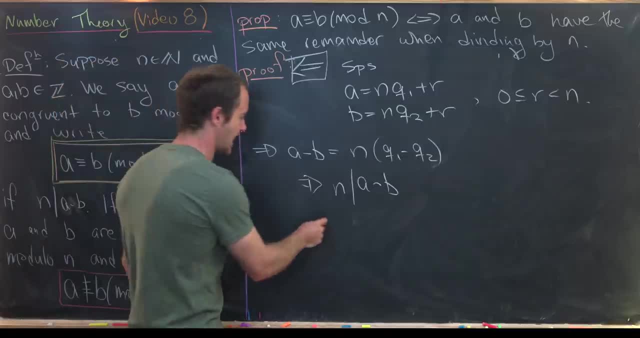 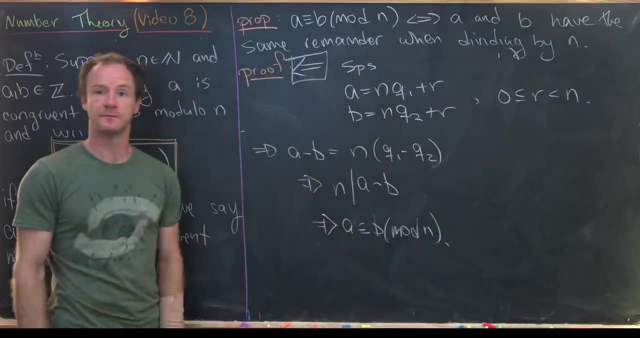 and now we're ready to prove that we have the same remainder when dividing by a minus b. But if n divides a minus b, then by our definition over here, a is congruent to b modulo n. And that finishes this proof. And now let's move on to our next result. Okay, next we'll prove a, really. 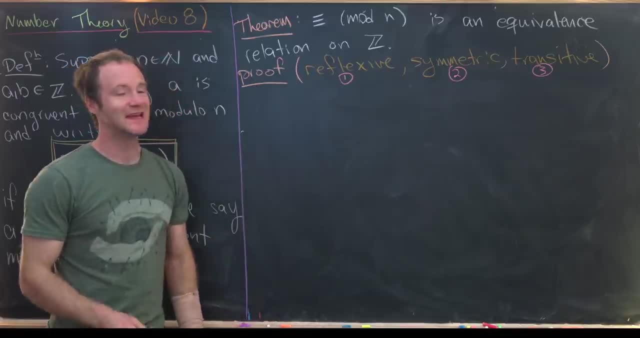 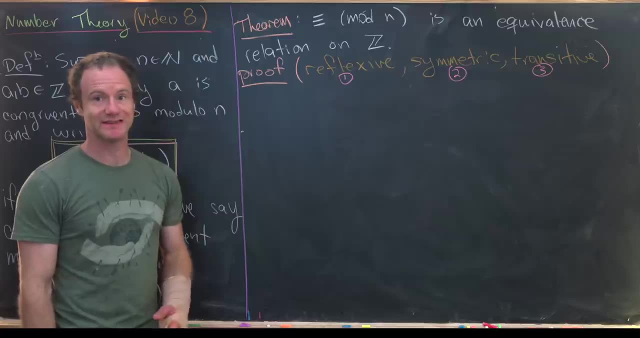 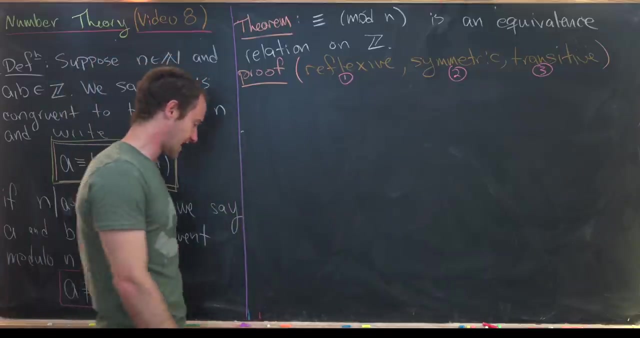 classic result that says that congruence modulo n is in fact an equivalence relation on the integers. So let's recall that an equivalence relation is a relation that these three properties: It is first reflexive, second symmetric and third transitive. So we'll 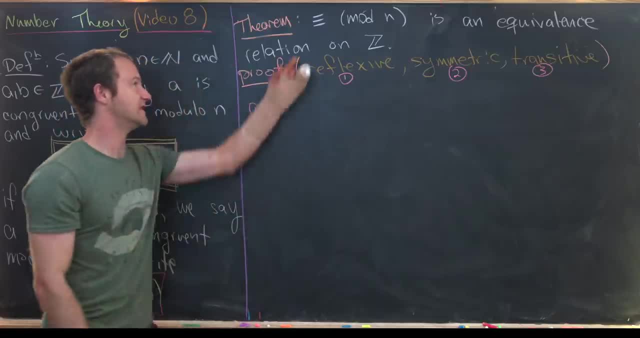 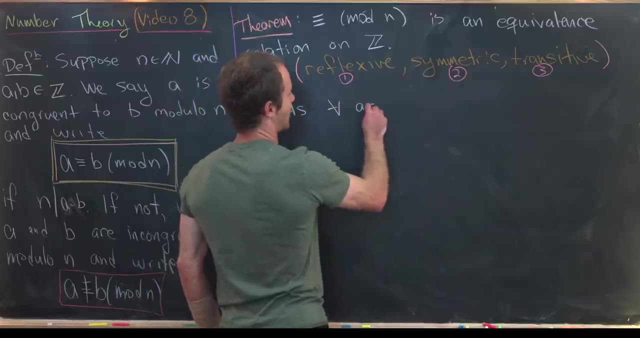 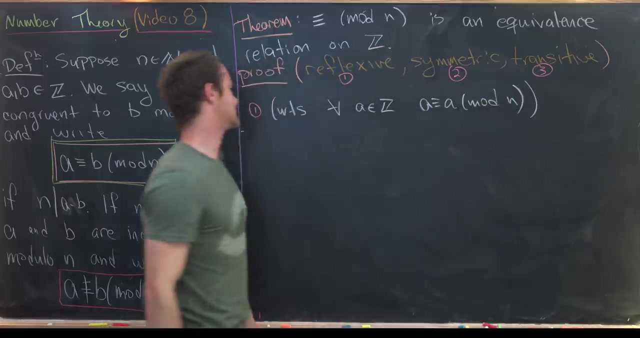 prove these one at a time. So let's first show that this relation is reflexive. So in other words, we want to show that for all a in z, a is congruent to a modulo n. That's what it would take to show that this thing is reflexive. But notice, this is most definitely true And we can. 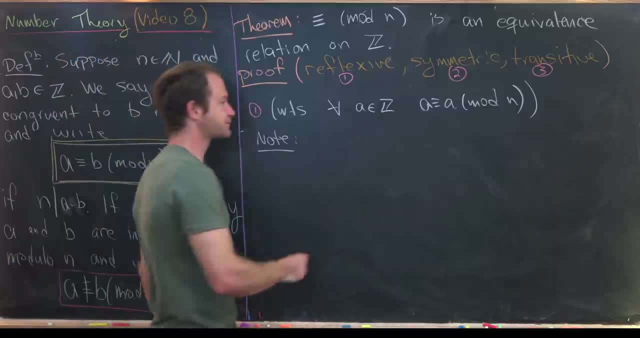 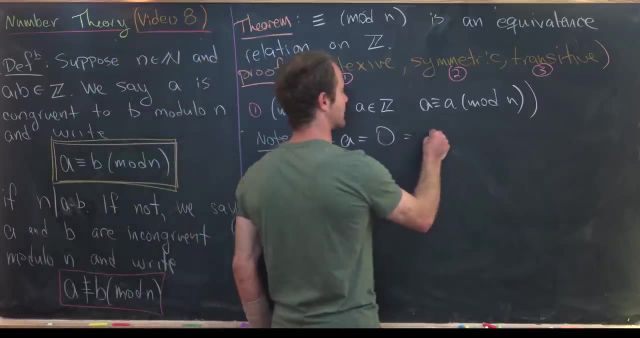 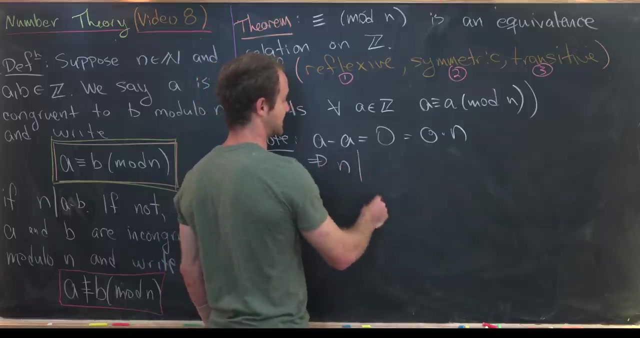 see that with the following like calculation: So let's notice that a minus a is equal to zero. Well, that's pretty obvious. But zero can be written as a multiple of n, as zero times n, But that tells us that n divides zero. but we can write zero as a minus a, But that's. 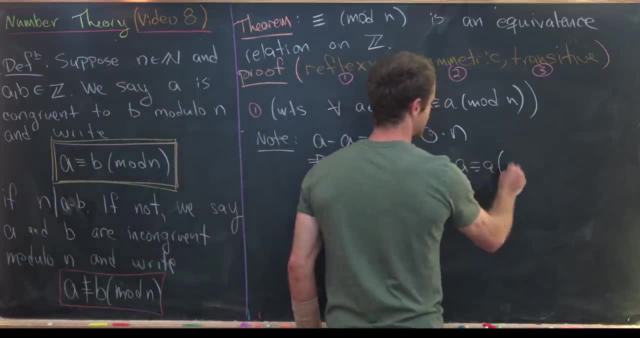 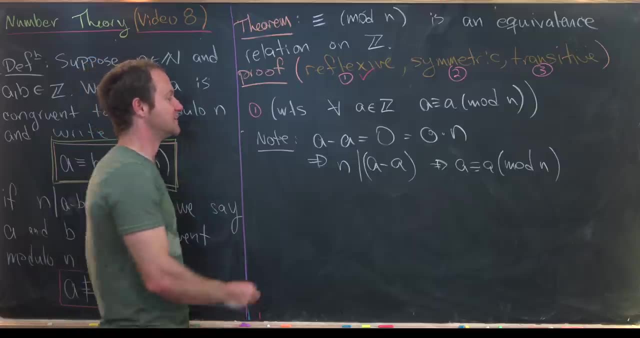 exactly what we want to show. So let's show that for all a in z, a is congruent to a modulo n. That's exactly the condition that we need for a to be congruent to a modulo n. So that means we've proven the reflexivity of this relation And now we're ready to prove the symmetry of. 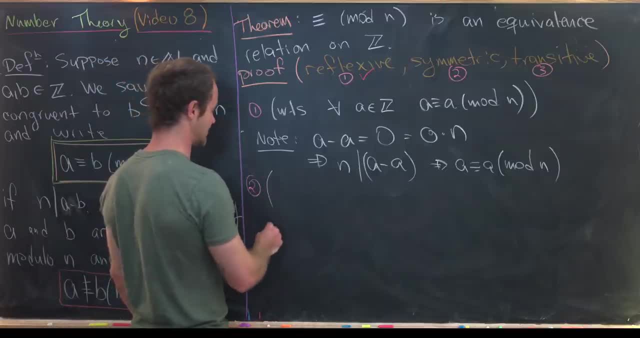 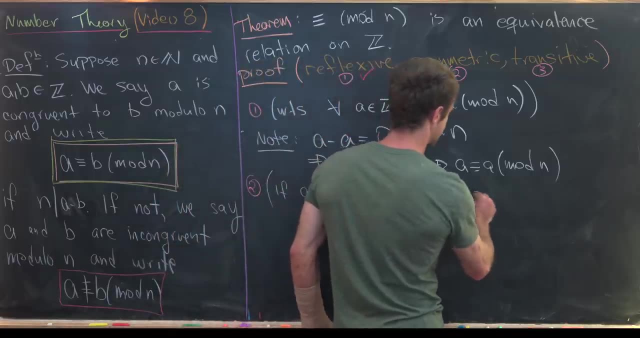 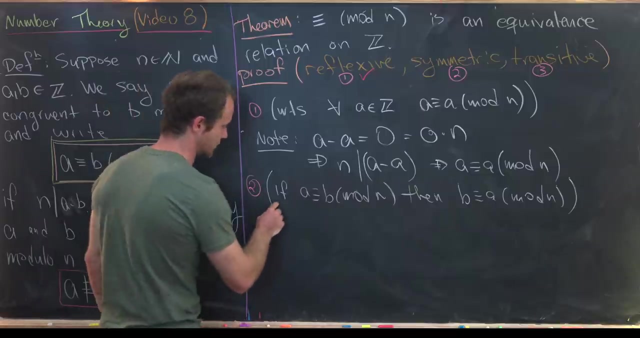 this relation. So let's recall that symmetry means that if a is congruent to b mod n, then b is congruent to a mod n. Great, So let's see how we can do that. So we'll start with one side of this proposition and prove the other side. So let's suppose that 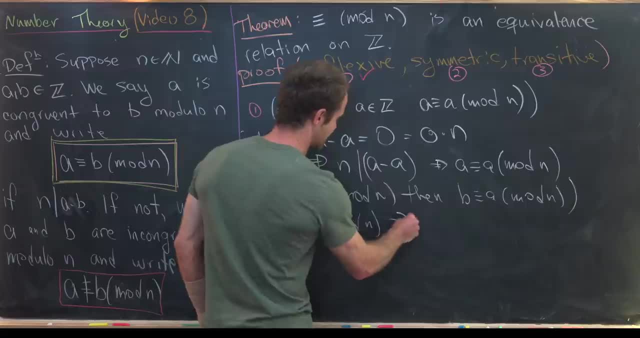 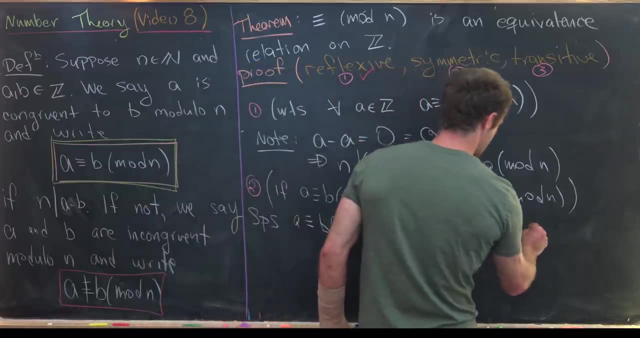 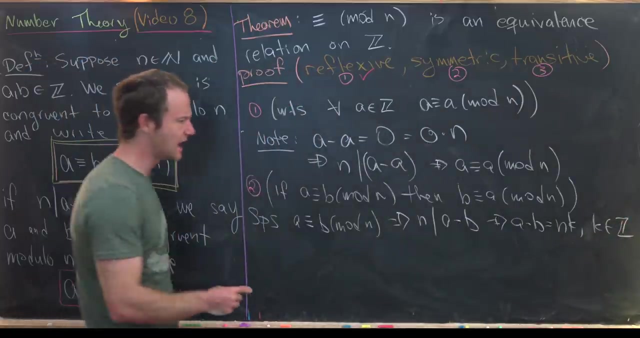 a is congruent to b mod n, But that tells us that n divides a minus b. But that means that a minus b is equal to n times k, where k is some integer. But that tells us that b minus a is equal to n. 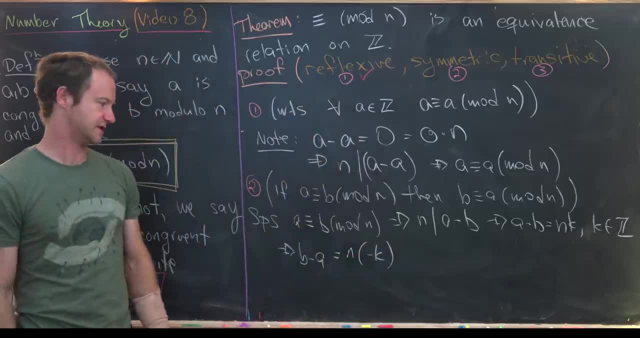 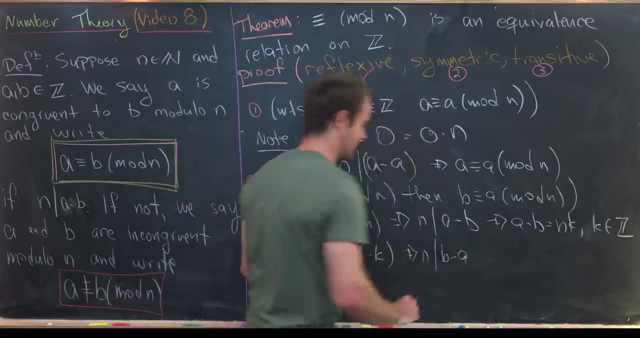 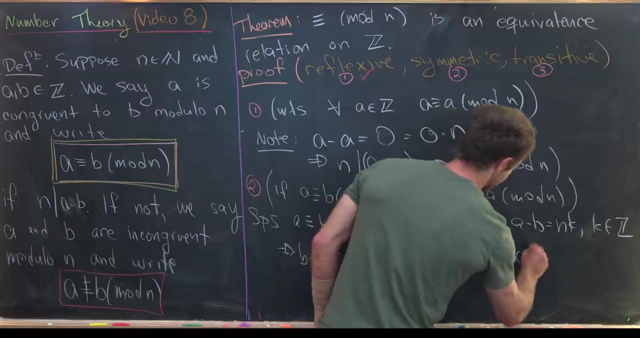 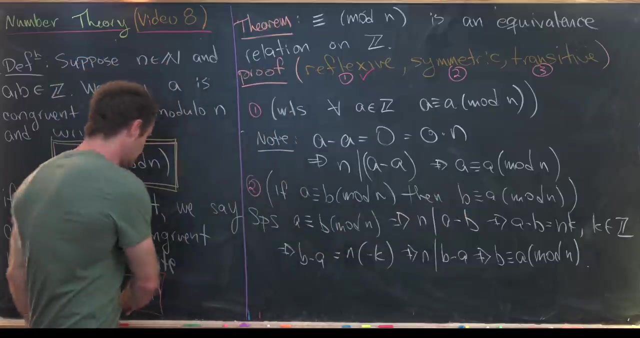 times minus k, just using arithmetic. But this is exactly the condition. we need to say that n divides b minus a. But if n divides b minus a, by our definition over here we have, b is congruent to a modulo n. So we started here and ended there. So that means we have just shown that. 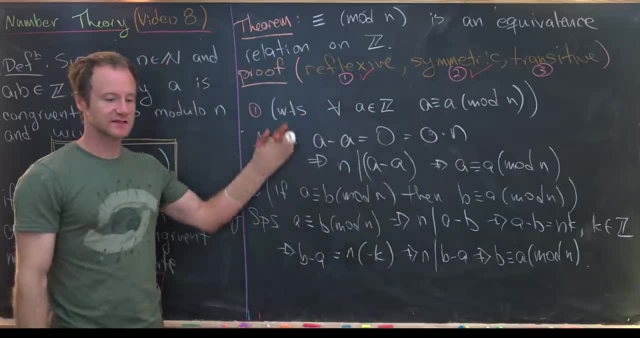 our relation is indeed symmetric. Now let's get back to the problem. So let's say that a is congruent to b- mod n and b is congruent to c- mod n. Now let's get rid of this and we will prove. 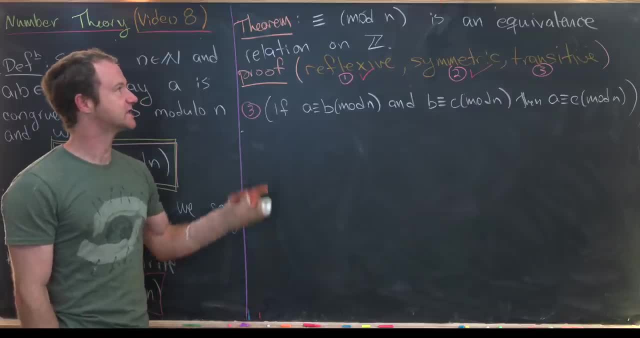 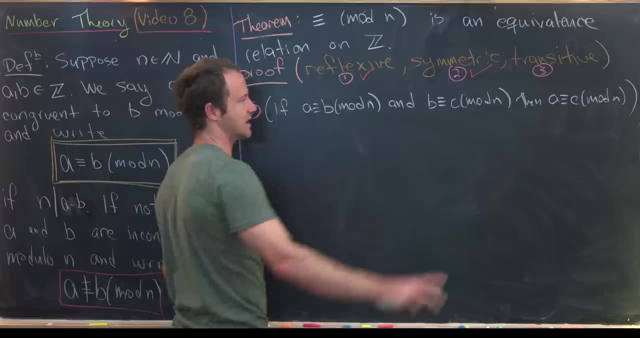 that it's transitive. So to finish this off, we need to show that our relation is in fact also transitive. So in other words, if a is congruent to b- mod n, b is congruent to c- mod n, then a is. 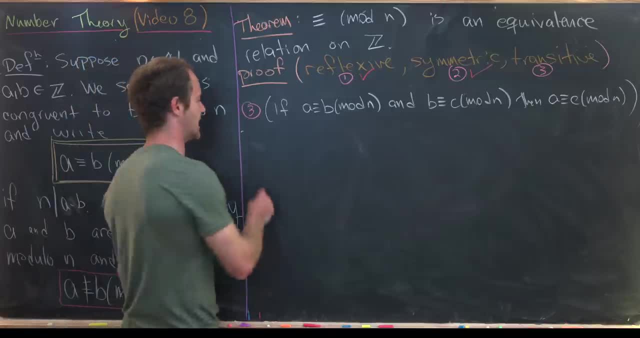 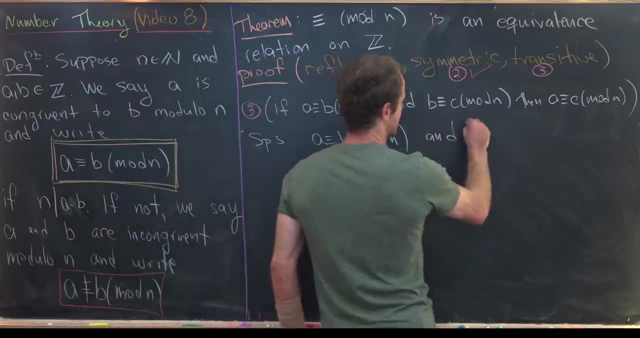 in fact congruent to c mod n. So let's maybe get to that. So we'll suppose first off that a is congruent to b mod n and b is congruent to c mod n. Now let's get rid of this and we'll prove. 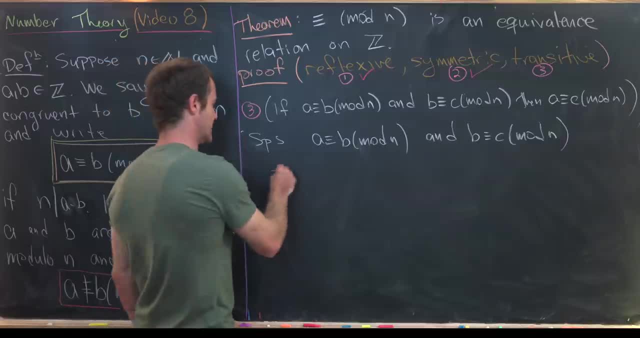 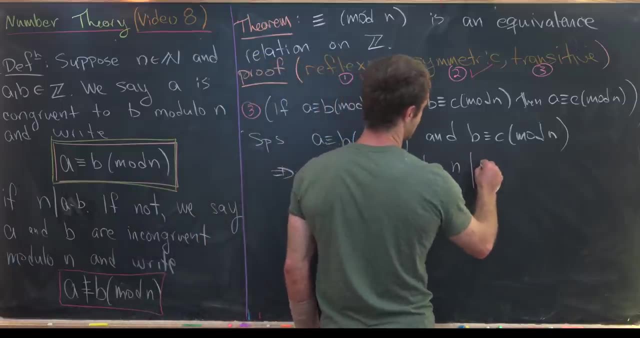 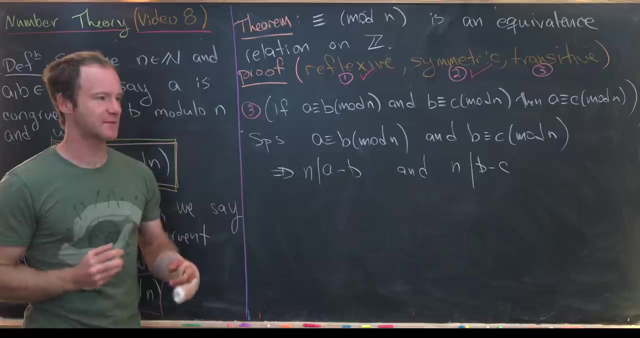 it. So let's unravel this via the definition of congruence: modulo n. So that tells us that n divides a minus b and n divides b minus c. Now we can actually jump to the end here, because we know something about divisibility and taking linear combinations. But instead of doing that, 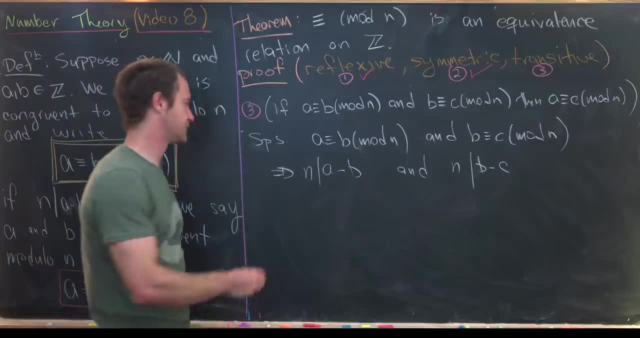 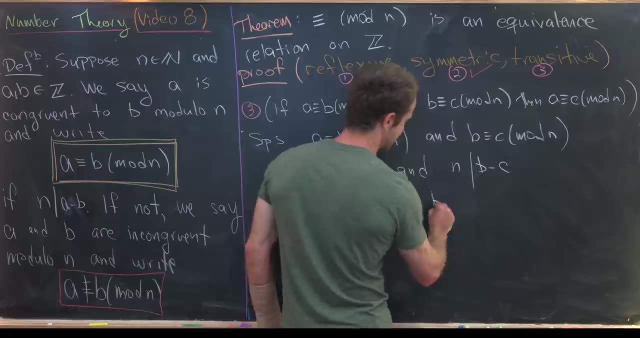 I'll put all the details in, just you know, because we can. Okay, so this means that a minus b is equal to n times k, and then this one over here means b minus c is equal to n times l, and this is for. 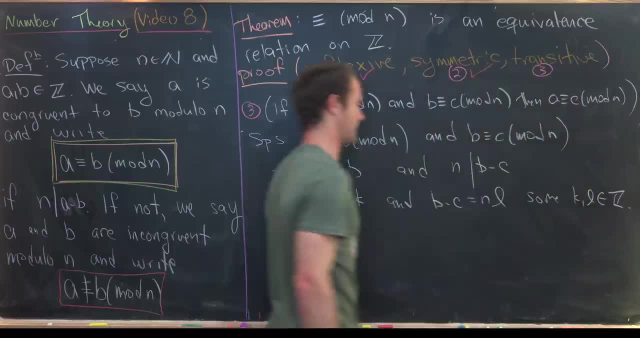 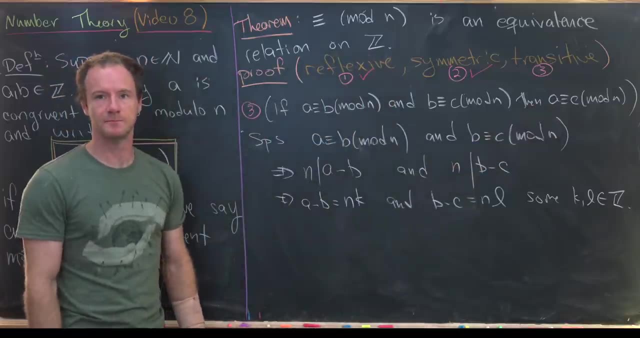 some integers, k and l. Okay, now let's look at what we're trying to get to. We're trying to get to: a is congruent to c mod n. That means we need to see something of the form a minus c. So how can? 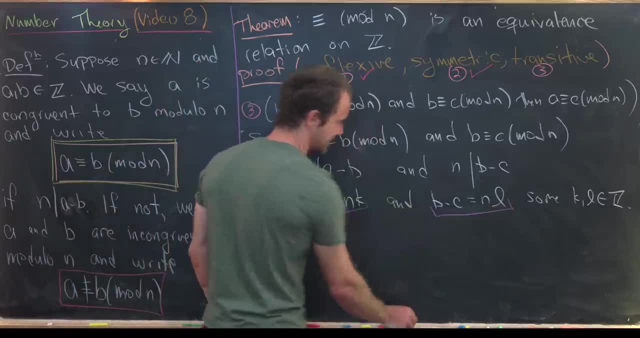 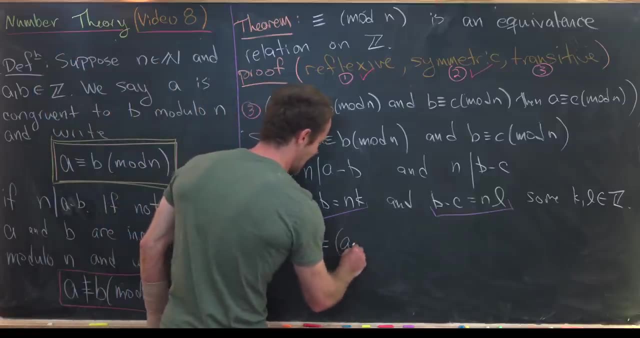 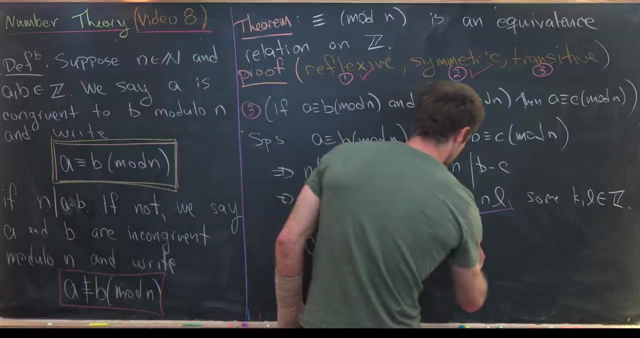 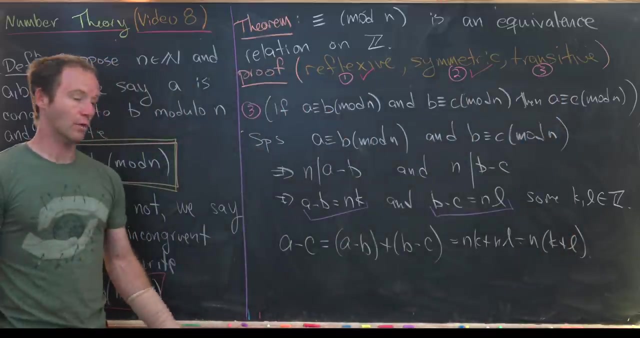 we do that? Well, we can do that by taking these two things, which I've underlined in purple, and adding them. So notice that a minus c is the same thing as a minus b plus b minus c, just by standard arithmetic. But that's also equal to nk plus nl, which is n times k plus l. But what do we have? 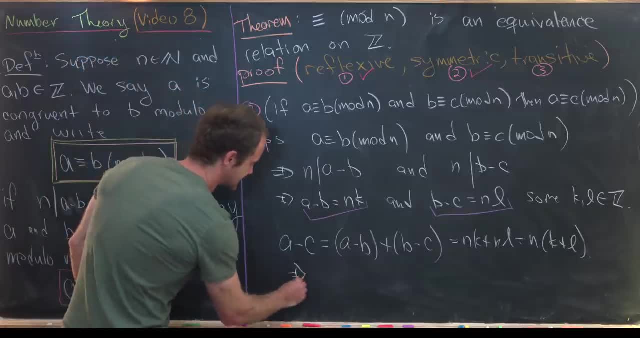 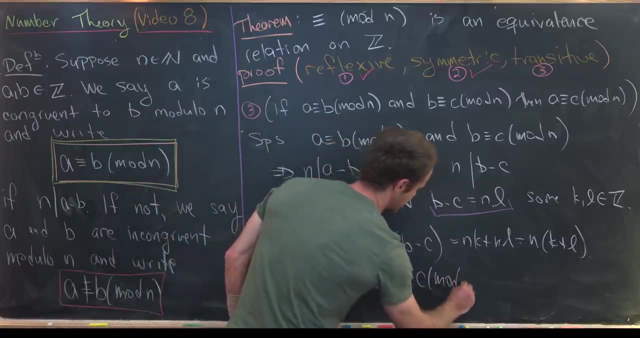 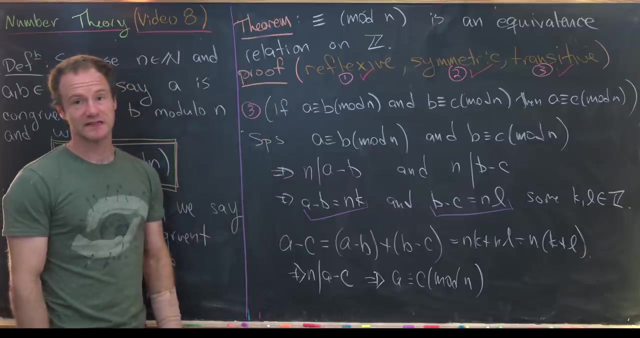 We have a minus c as a multiple of n. That means that n divides a minus c, but that means that a is congruent to c modulo n And that finishes off this proof that our relation is in fact transitive. So that means it's. 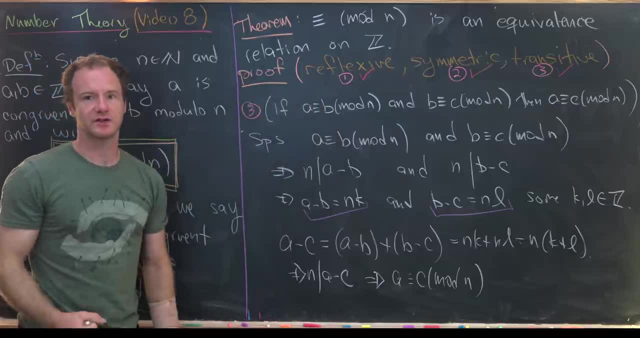 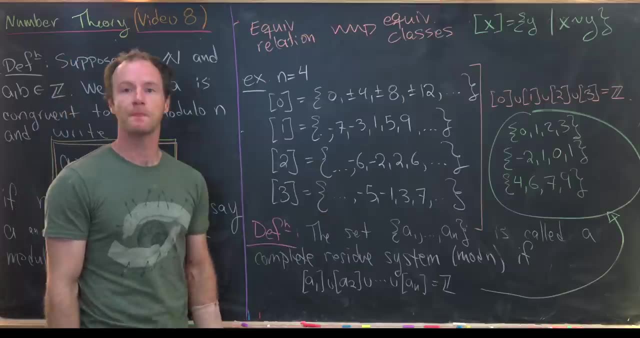 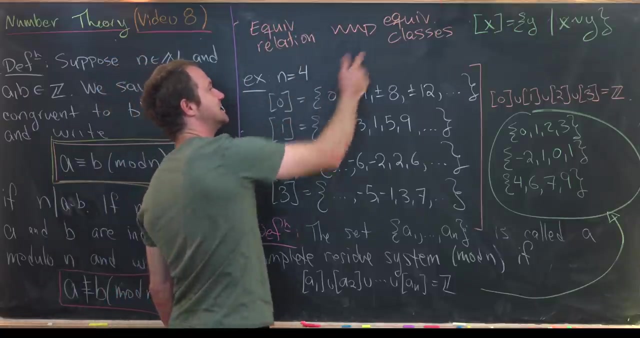 reflexive, symmetric and transitive, which means congruence. modulo n is, in fact, an equivalence relation on the integers. Okay, so now let's move on. Before we move on to our next result, I want to recall that the notion of an equivalence relation leads to the notion of an equivalence. 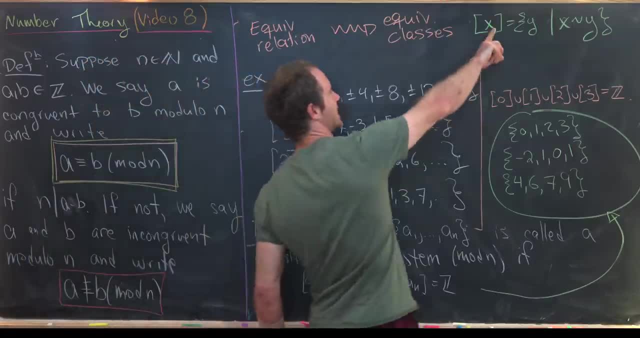 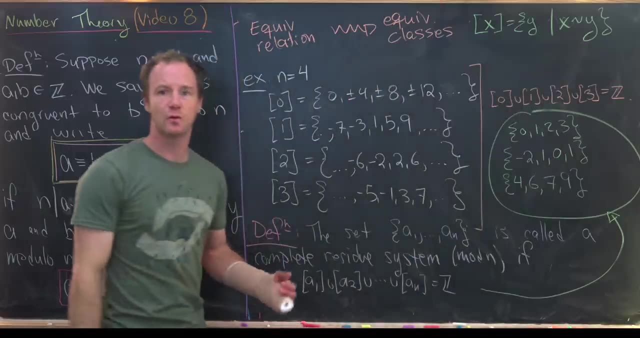 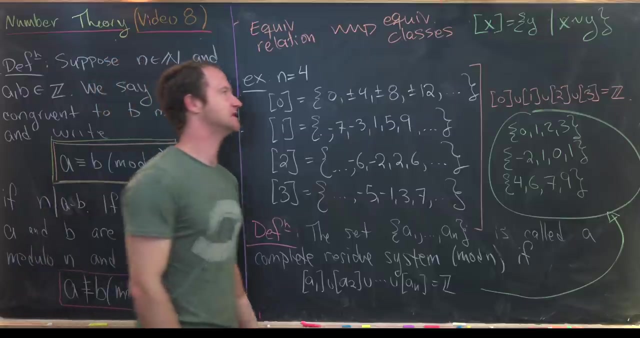 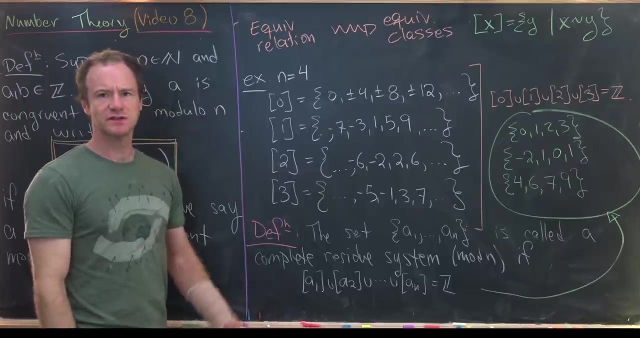 class. So the equivalence class of the element x is all elements y that are equivalent to x under whatever equivalence relation that you're working with. So here we're working with congruence modulo n. So that means we would read this as all y, which are integers, where x and y are congruent modulo n. So let's look at some examples. 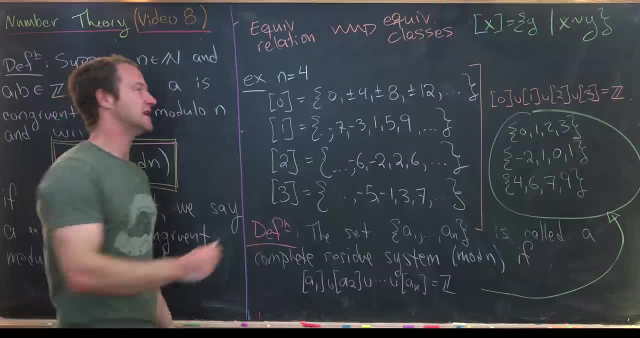 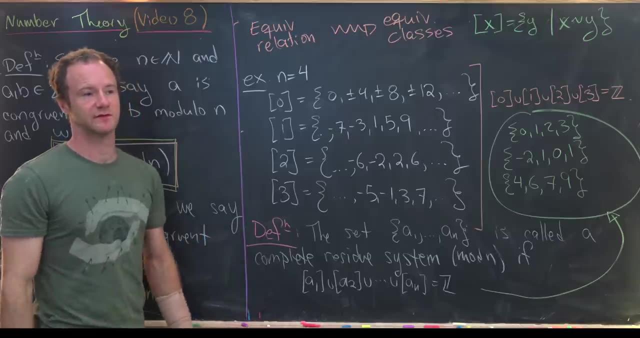 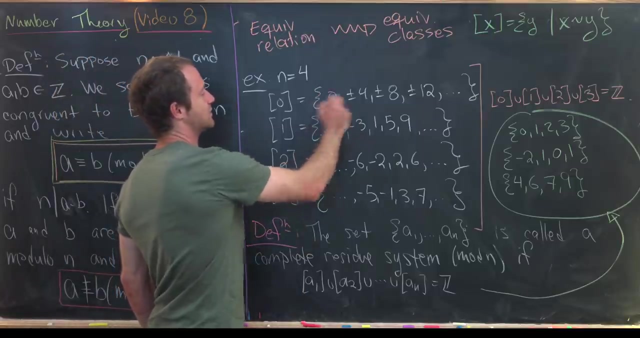 So n equals four. the equivalence class of the number zero is everything congruent to x. So that's a to 0 mod 4.. In other words, all multiples of 4.. Because we can think about just keeping the remainder after dividing by 4.. So that means we've got 0 plus minus 4, plus minus 8 plus minus 12 and 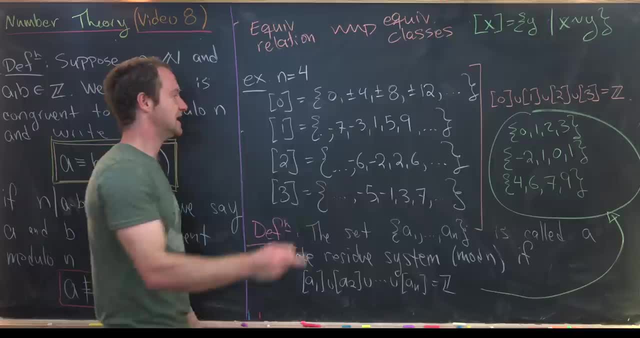 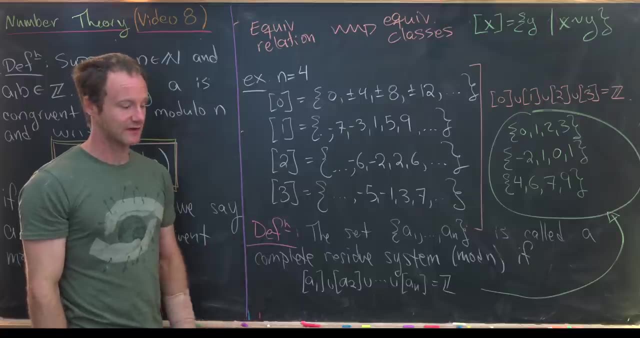 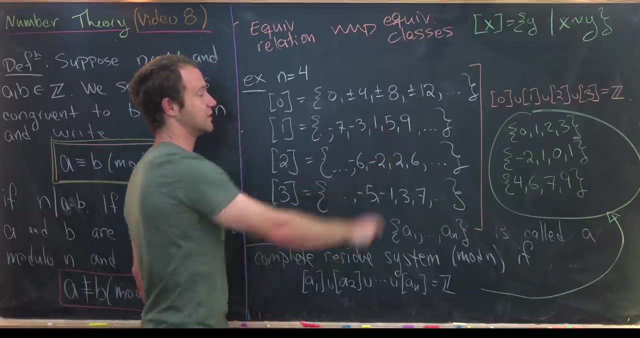 so on and so forth. That's the equivalence class. Next, the equivalence class of 1 is everything that's congruent to 1 mod 4. In other words, everything that has a remainder of 1 after dividing by 4.. So 1,, 5, 9, so on and so forth in that direction, And also back in the other. 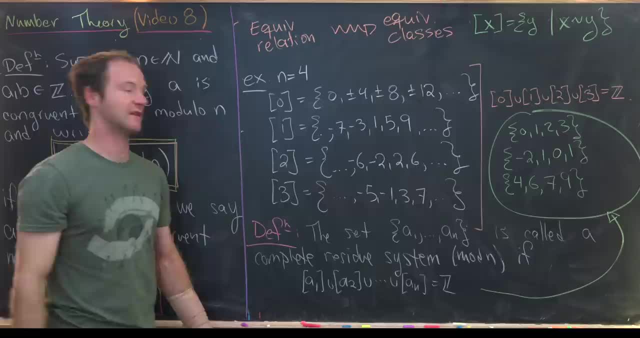 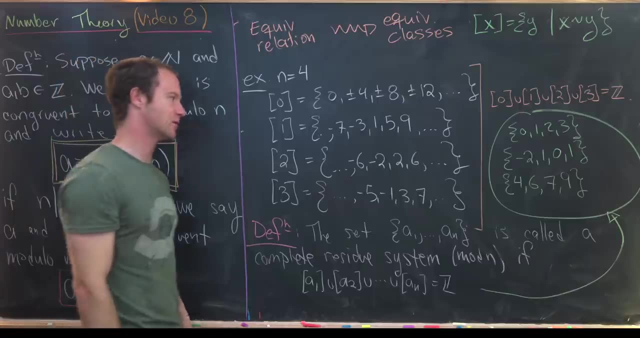 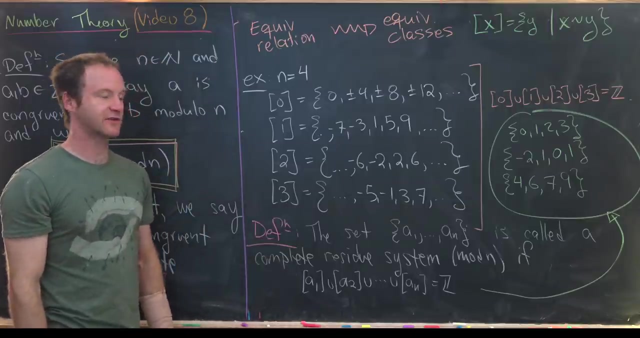 direction. So minus 3,, minus 7, and so on and so forth in the negative direction. Next, the equivalence class of 2 is everything that has a remainder of 2 when dividing by 4.. So we've got minus 6,, minus 2,, 2, 6, and so on and so forth. Finally, the equivalence class of 3 is everything. 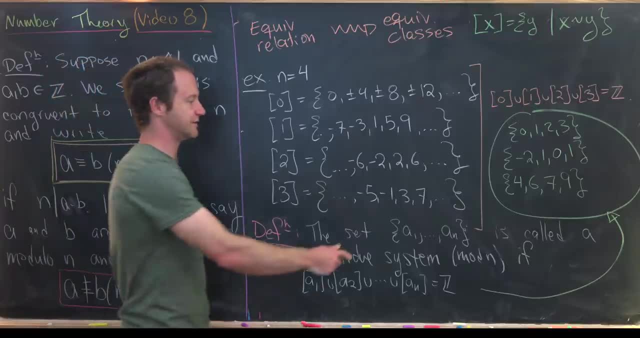 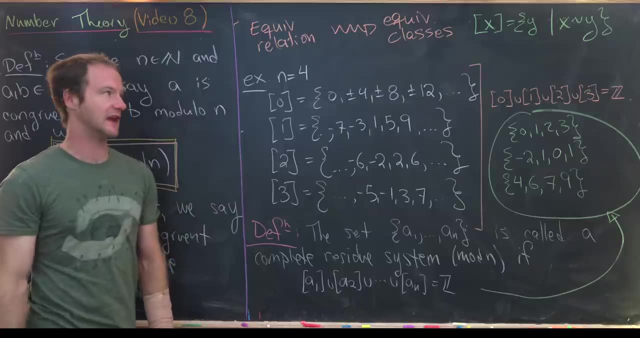 that has a remainder of 3 when dividing by 4.. So we've got like 3,, 7, and then so on and so forth in that direction: Minus 1,, minus 5, and then back in the negative direction as well. So I want to notice that if we take these four, 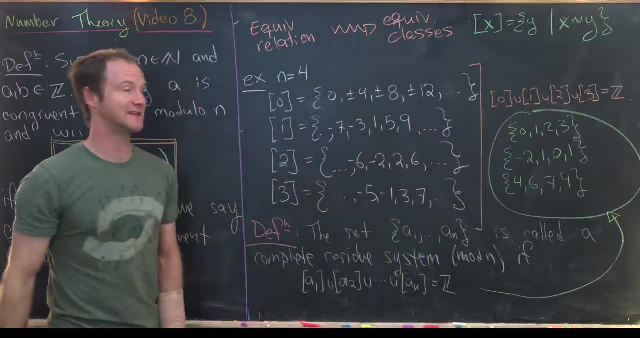 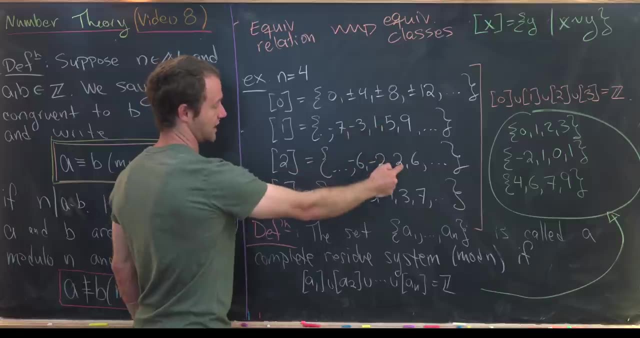 equivalence classes 0,, 1,, 2,, 3, and 4, and take their union, then we get all of the integers. So notice, we can count those up: 0,, 1,, 2,, 3,, 4,, 5,, 6,, 7. And you can see that we'll get all the. 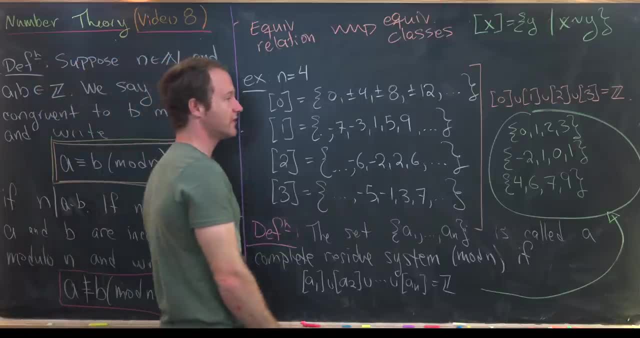 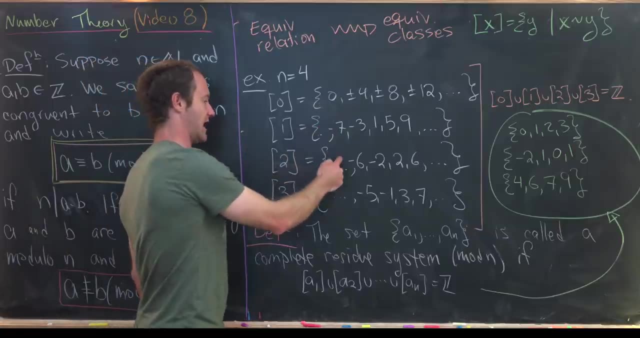 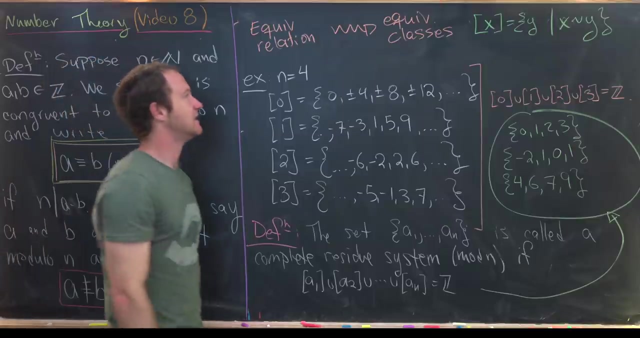 integers. Now, another thing that I want to notice is that these are, in fact, disjoint unions, In other words, there's no overlap between these equivalence classes. That's a standard result that you probably saw in an intro to proofs class that an equivalence relation, and equivalence classes. 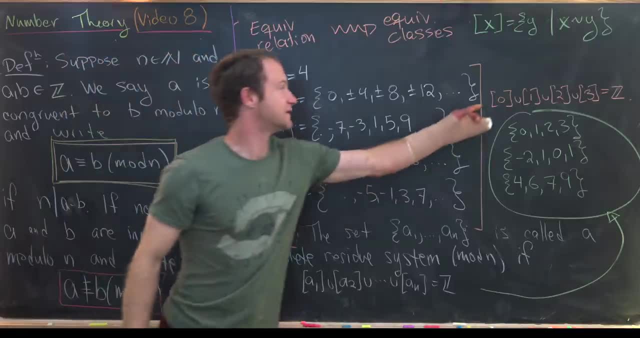 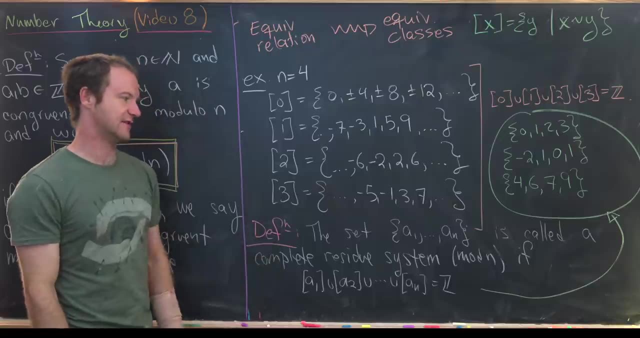 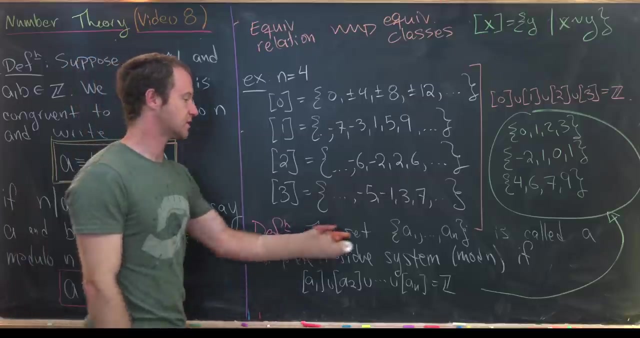 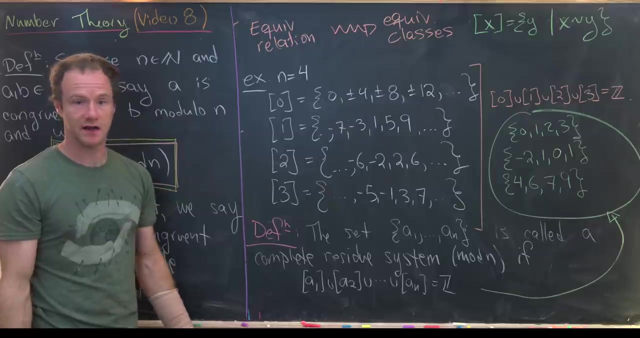 lead to a partition of a set. So in fact we've got a partition of the integers into four sets there. Okay, that leads us to a another definition, And that's the definition of something called a complete residue system- modulo n. So the set of integers a1,, a2, up to an is called a complete residue system, mod n. 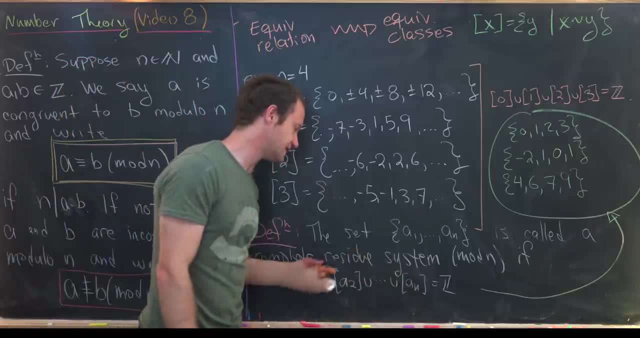 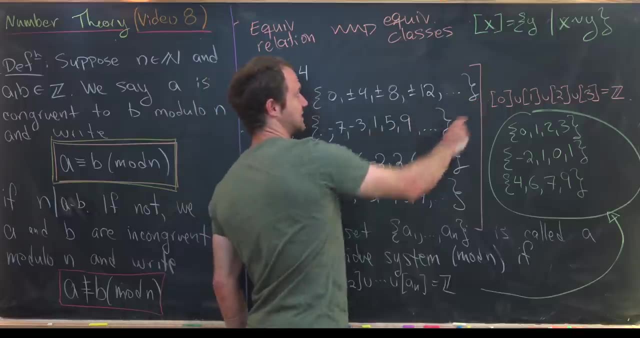 if, when we take the union of these n equivalence classes, we get all of the integers. So from our original example up here we see that 0,, 1, 2, 3 make a complete residue system modulo n, And that's the definition of something called a complete. 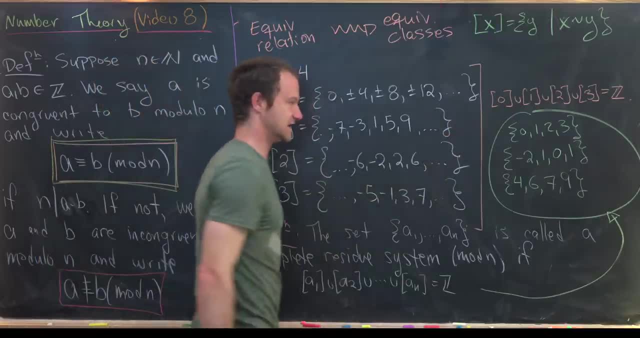 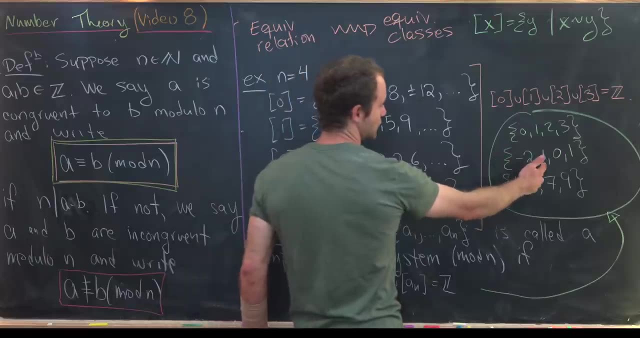 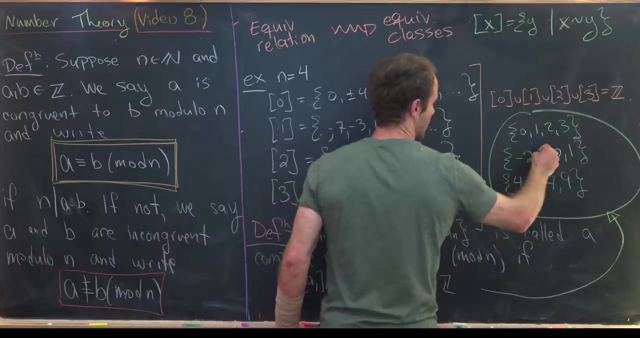 residue system And that's because these union to the integers. But we could take other equivalence class representatives if we wanted to So notice that negative 2, 1, 0, 1,- sorry, negative 2,, that should be negative 1, 0, 1, also form a complete residue system And that's again. 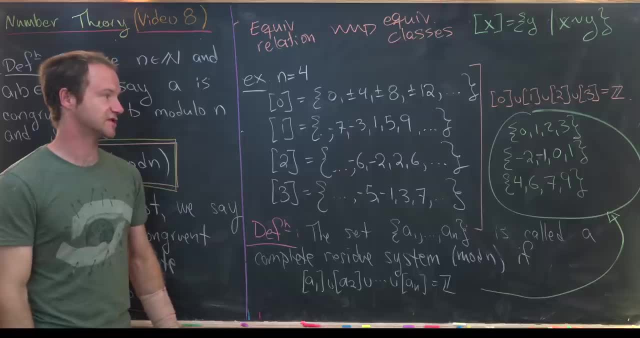 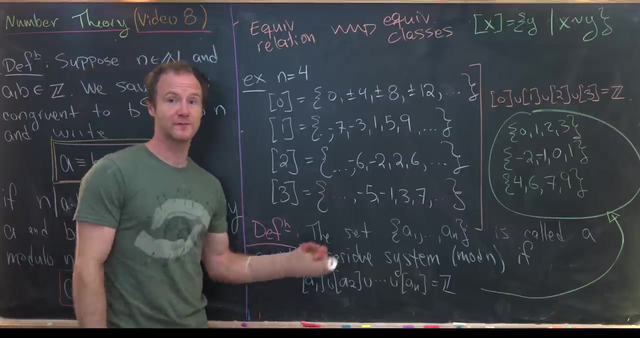 because their equivalent classes will union to the integers. Similarly, 4,, 6,, 7,, 9, that's another kind of strange complete residue system. Okay, so let's maybe get rid of this, And then we'll prove the relationship between basic arithmetic and congruence modulo n. Now we're going to prove. 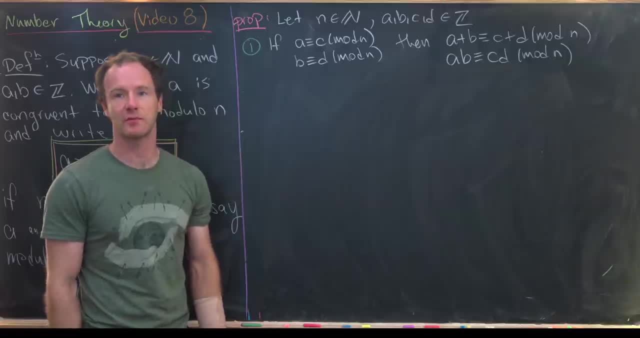 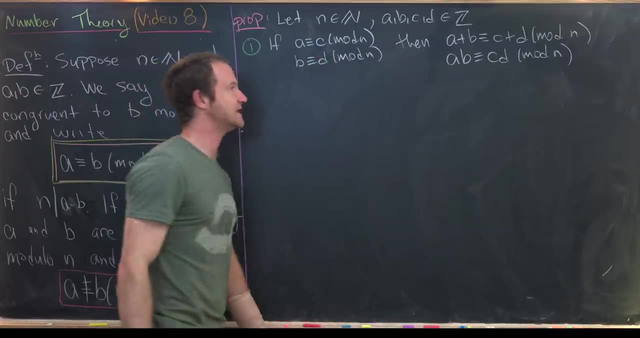 a. four part proposition involving the arithmetic properties of congruence modulo n. Starting with the following setup: we've got a natural number, n, and a, b, c and d are integers. Furthermore, we're assuming that a is congruent to c mod n and b is 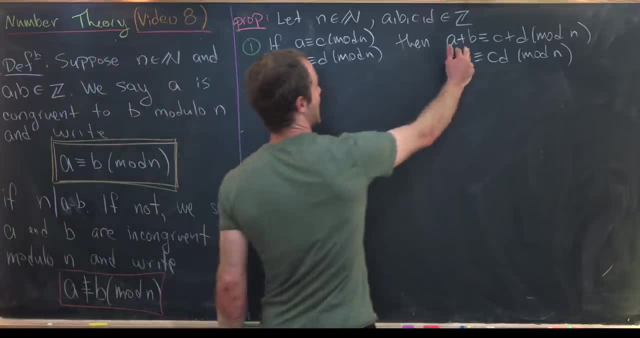 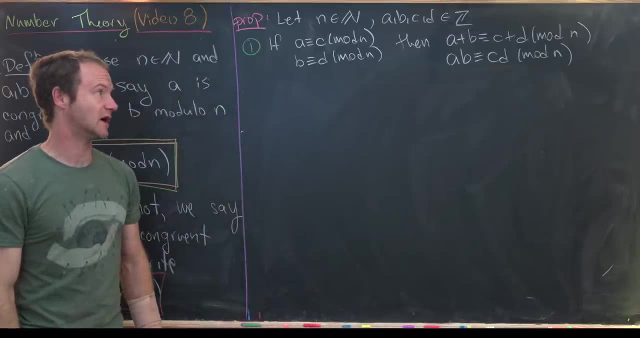 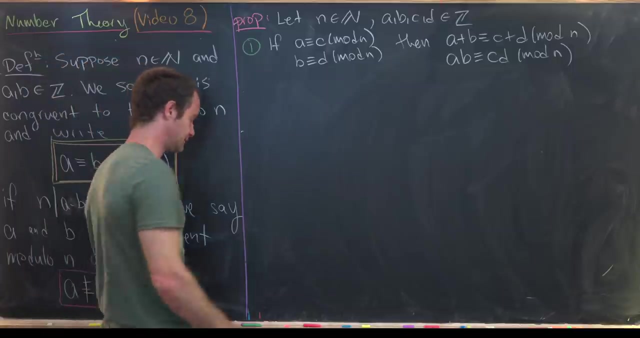 congruent to d mod n, Then it will follow that a plus b is the same thing as c plus d mod n, and a times b is the same thing as c times d mod n. In other words, this addition and this multiplication are well-defined modulo n. Okay, so let's maybe see how we can prove this first bit of the. 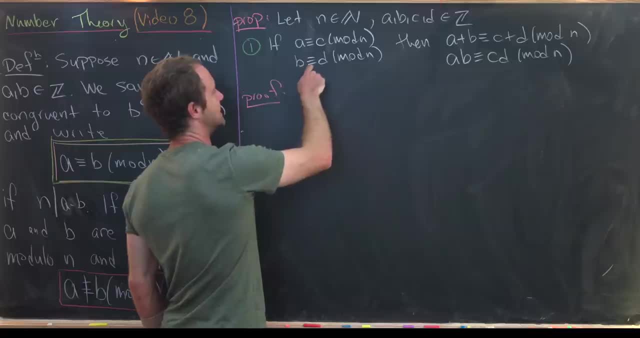 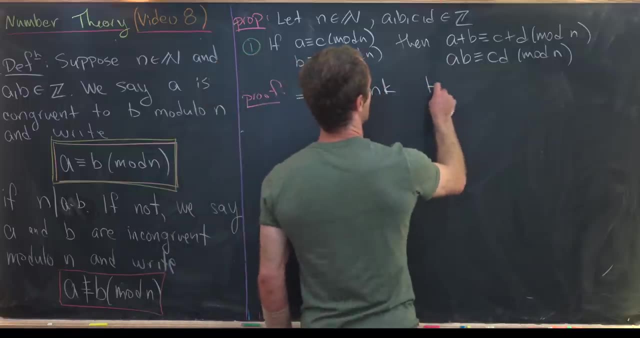 proposition. So notice that a is congruent to c, b is congruent to d, So that means that a minus c is equal to n times k, and b minus d is equal to n times l, where k and l are some. 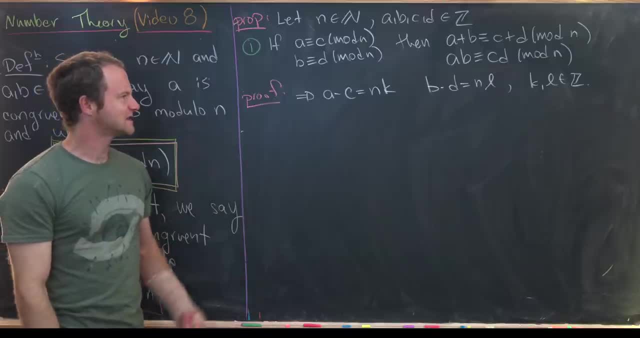 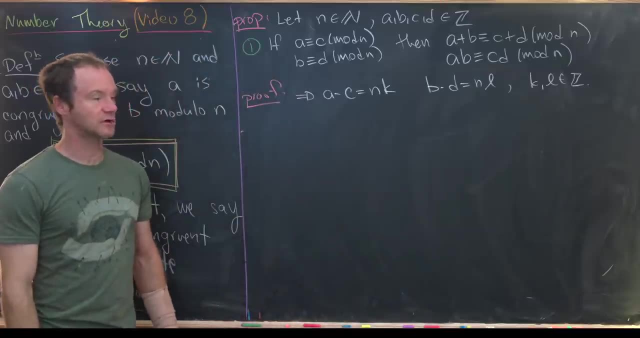 integers. Okay, now let's see where we want to go. We want to look at this a plus b and this c plus d, But for those to be congruent, modulo n, we need to discover their difference. So let's see how we 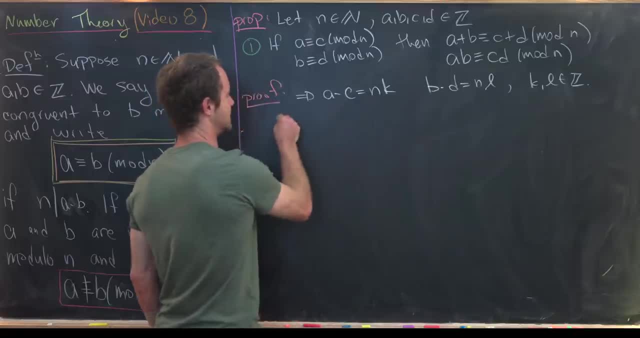 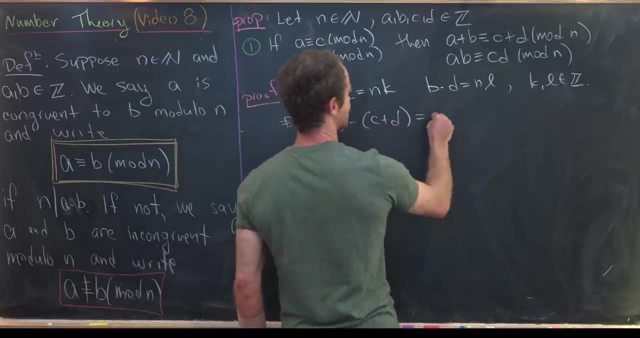 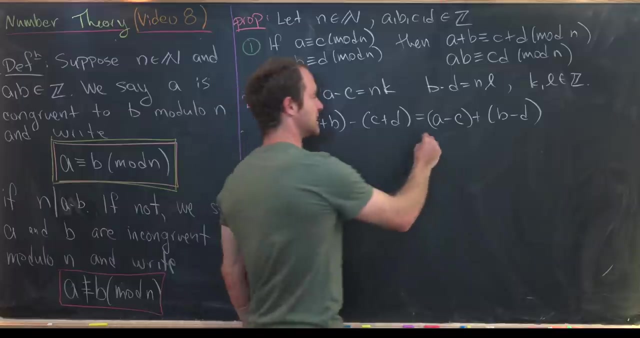 can do that. Well, we can get their difference by adding these two equations. So notice that a plus b minus c plus d is the same thing as a minus c plus b minus d, just by normal arithmetic rules. But that's the same thing as n k plus n l. 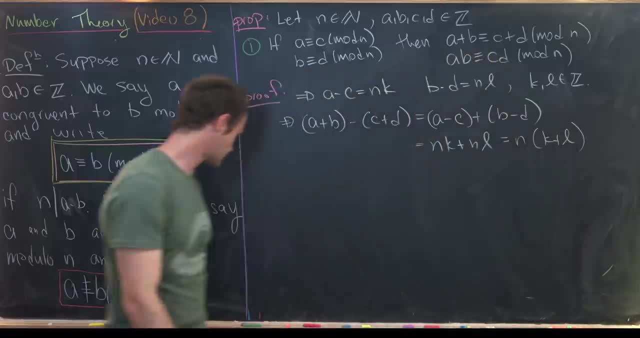 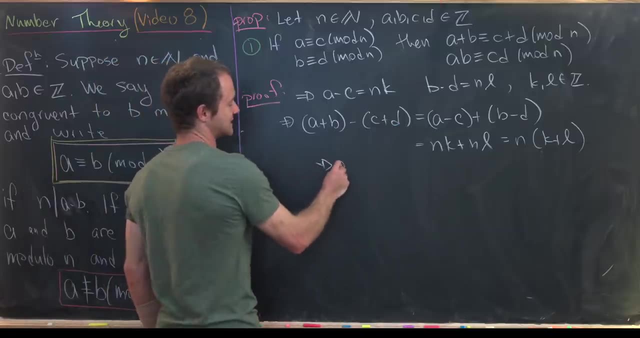 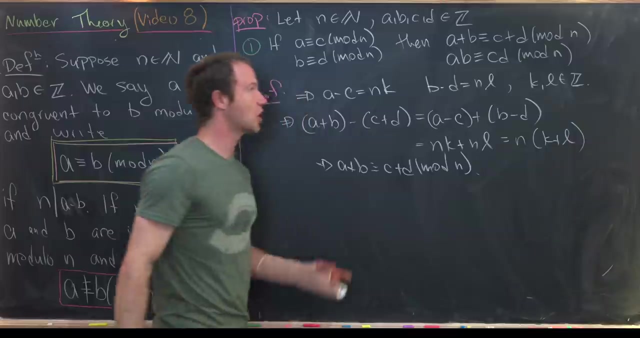 which is the same thing as n, k plus l. But what do we have? We have a plus b minus c plus d is a multiple of n, but that's the same thing as saying that a plus b is congruent to c plus d modulo n, as we were going for in this first part. Okay, now let's look at multiplication. 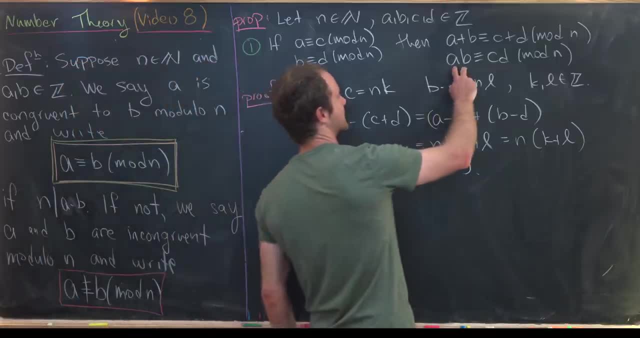 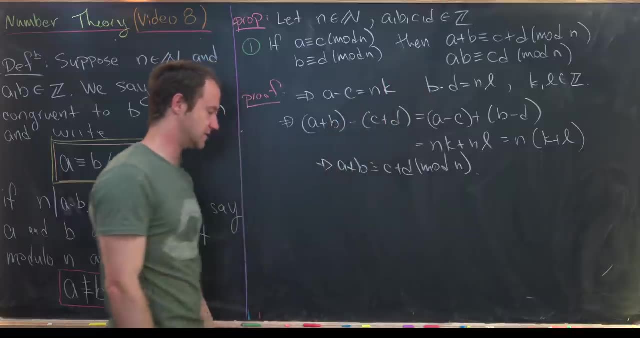 So for multiplication, we're trying to look at the product of a and b and the product of c and d. Well, we could get at that just by multiplying these two, but it's going to be useful to rewrite them a little bit. So let's do that. Let's notice that these two equations can be easily rewritten. 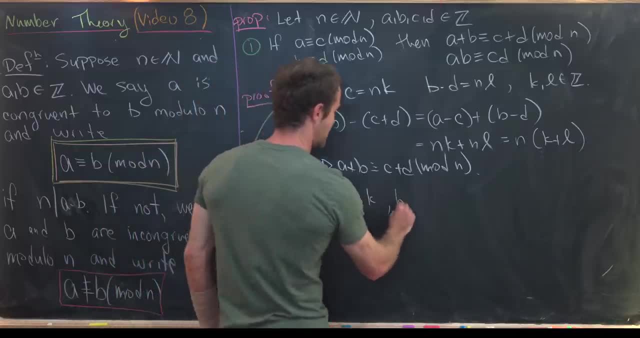 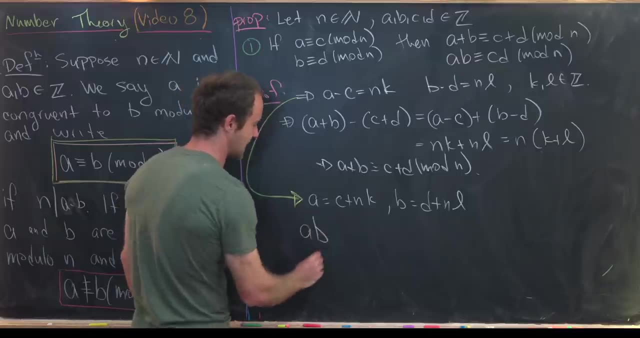 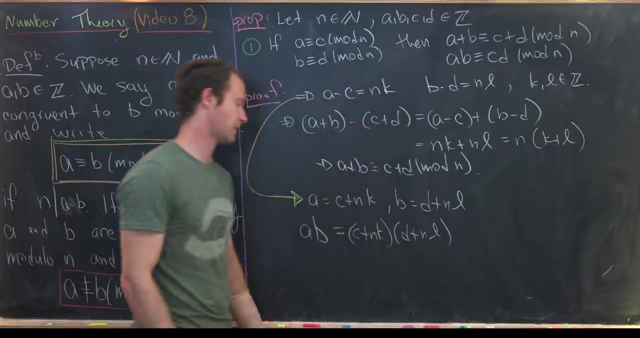 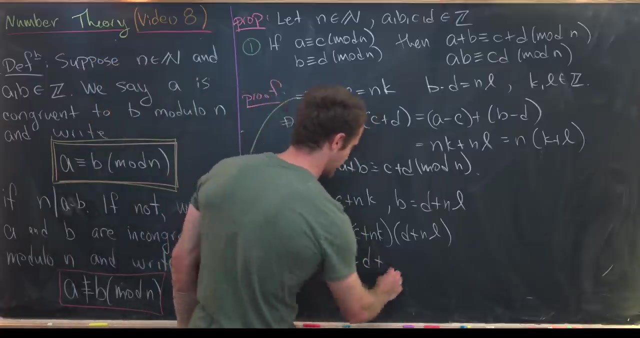 together by연 rę mallene. c plus n? k or c plus n k. times d plus n? l. Now we can multiply these. Notice that a times b equals c plus n k. times d plus nl. Now we can foil out that right hand side, leaving us with cod plus. what do we have? n times a bunch of stuff. So we're going to have cl times n2 and carbon times l. 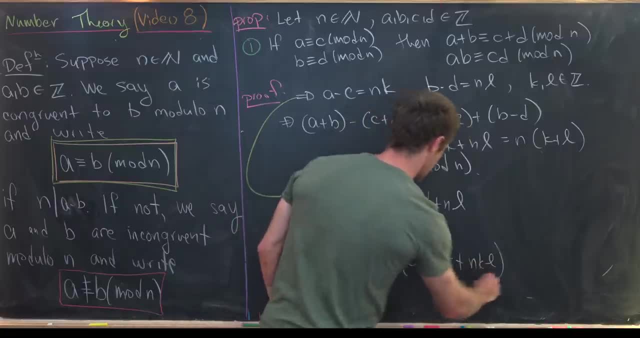 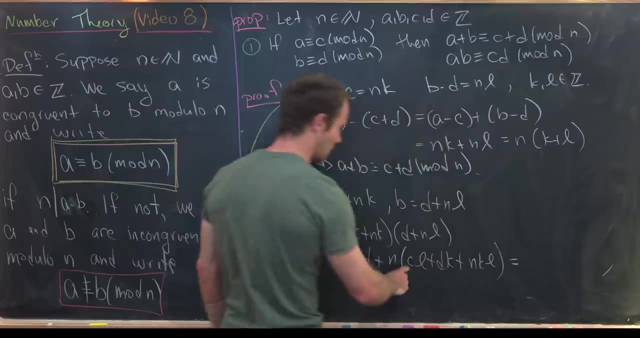 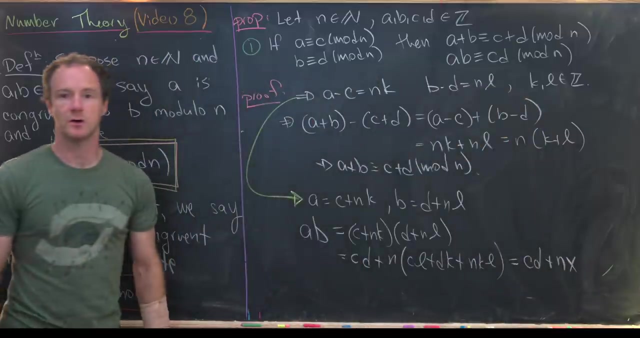 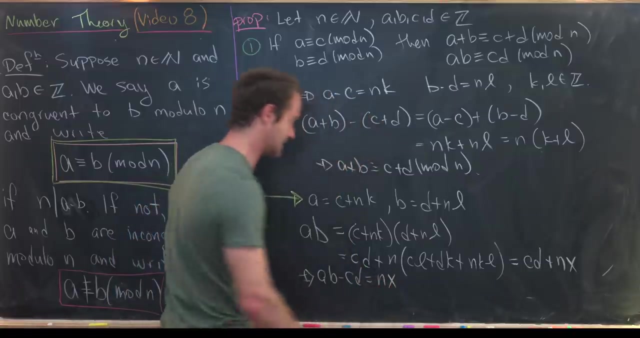 plus dk plus nkl. The important thing is that we've got n times something, So I'm just going to put these all together into the number x We have. this is equal to cd plus nx. Okay, but notice that tells us that ab minus cd is equal to n times x. In other words, 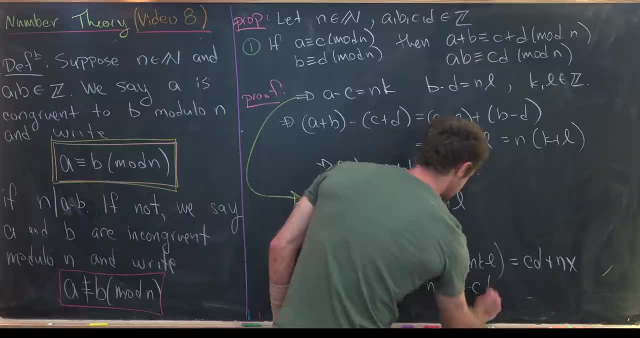 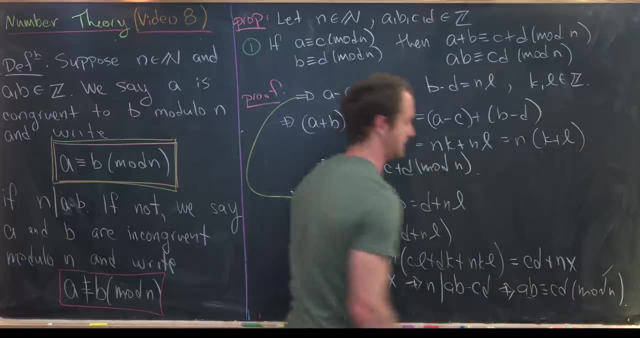 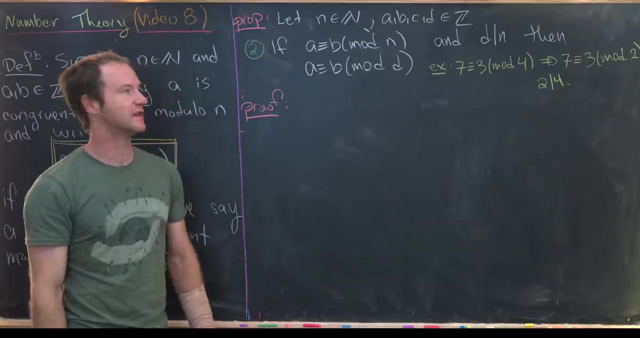 n divides ab minus cd, which is exactly what we need for ab to be congruent to cd modulo n. Okay, now that we've gotten this taken care of, let's move on to the second part of this proposition. Now we're ready to move into the next part of our proposition. Here we're going. 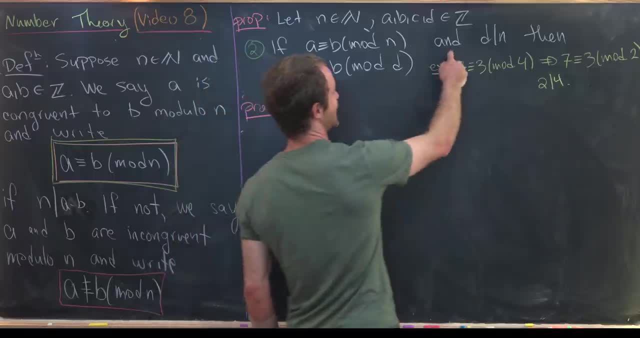 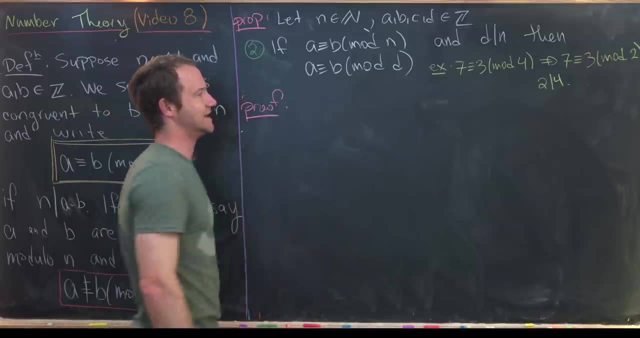 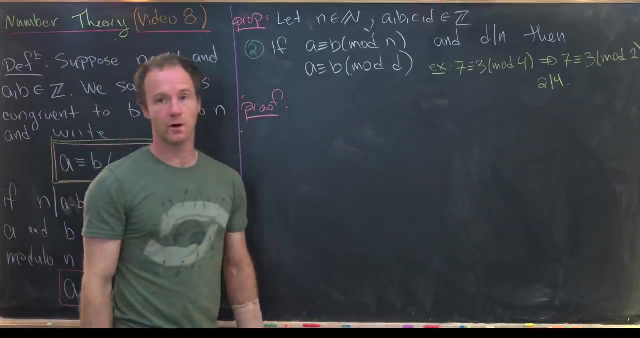 to assume that a is congruent to b mod n and d divides n, Then it will follow that a is congruent to b mod d. So let's look at a little example of that. So notice that 7 is congruent to 3 mod 4. 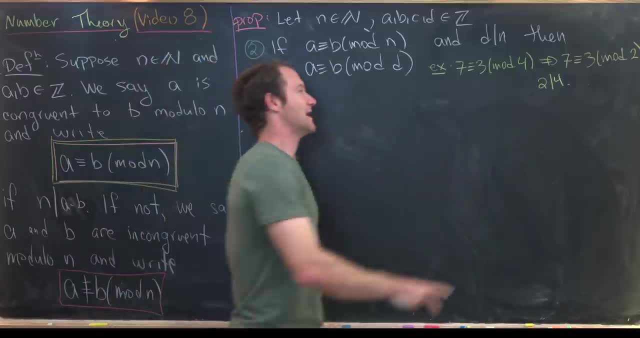 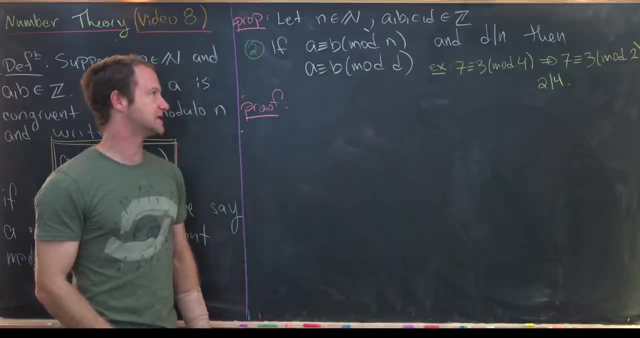 and 2 divides 4.. Well, that means that 7 will be congruent to 3, mod 2.. Okay, so let's maybe jump into the proof now. So by the fact that a is congruent to b, mod n, that means we can write. 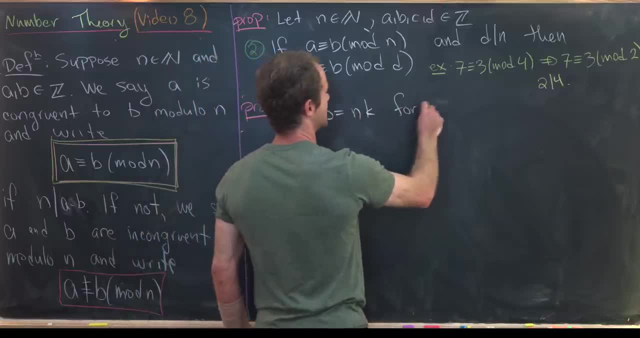 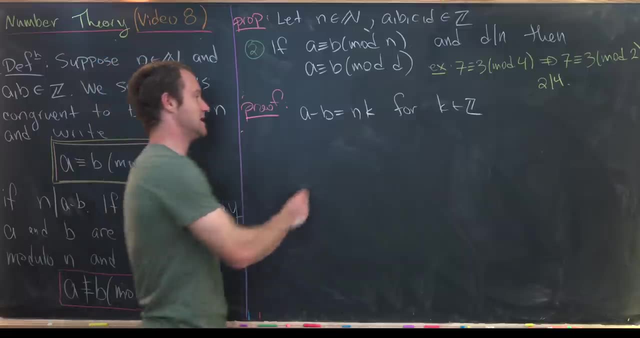 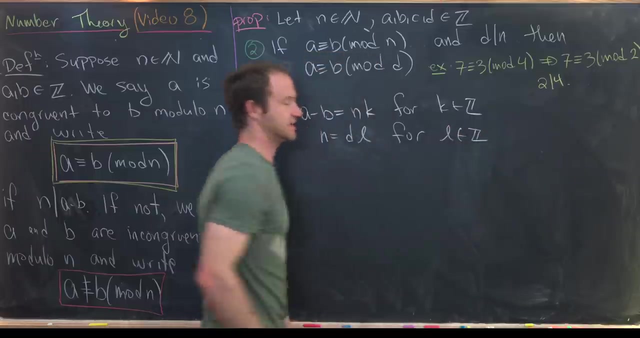 a minus b as n times k for some integer. Okay, and then from the fact that d divides n, that tells us that n is equal to d times l. for some, l, which is an integer, And I guess I should say l here is more strictly, a natural. 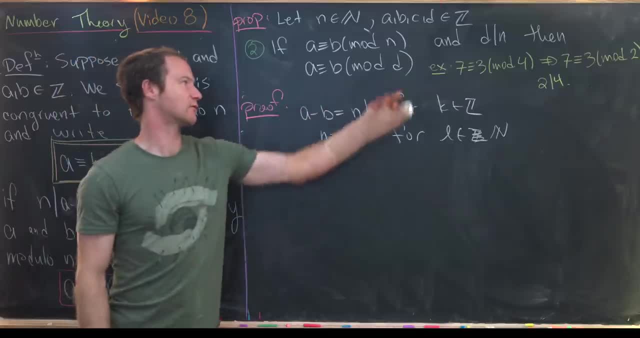 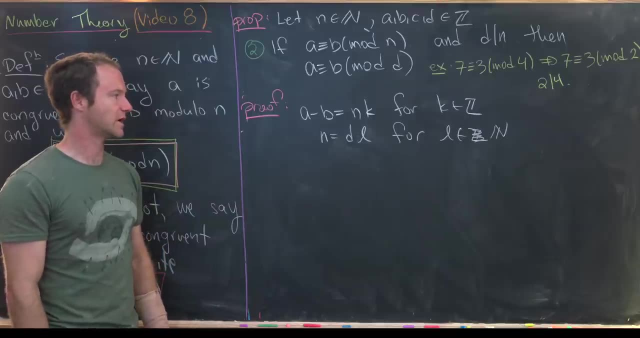 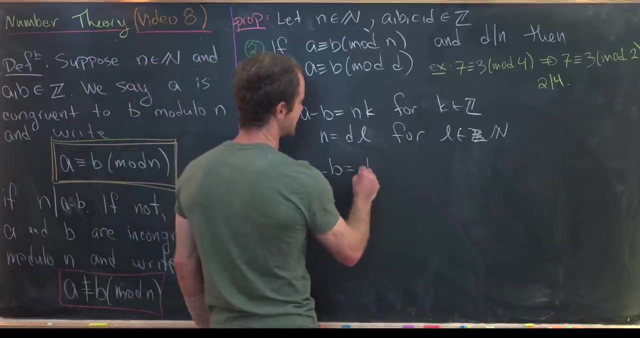 number and that's built into the context that we're reducing modulo d and that reduction modulo d really only works if we've got a natural number there. Okay, great, Now we can smash these two together and we'll see that a times b is equal to d times lk, But that means that d divides. 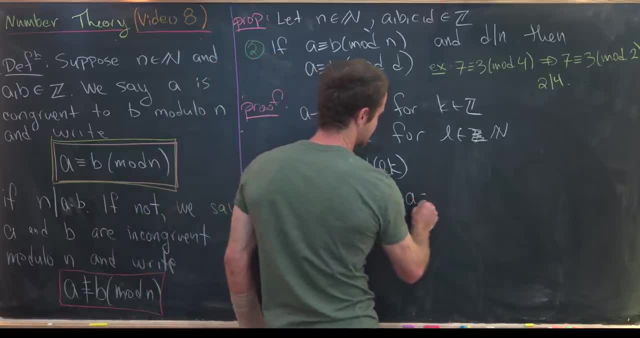 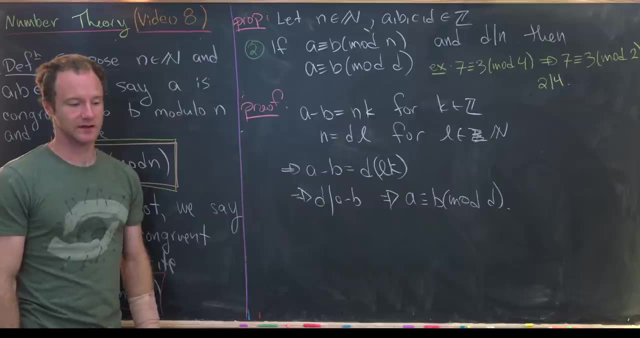 a minus b, which tells us that a is in fact congruent to b mod d, which is exactly what we wanted to get at for this second bit. Okay, so now let's move on to the third. Okay, the next bit of. 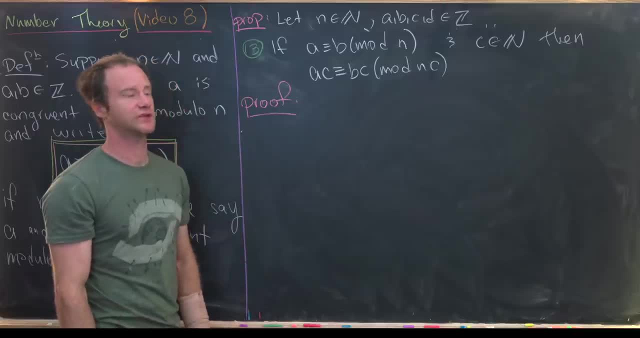 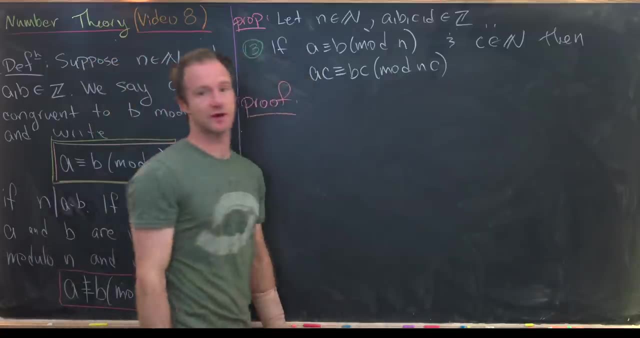 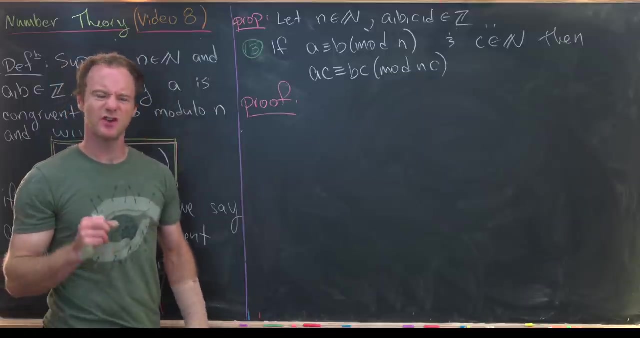 this proposition looks a little bit like the converse of what we just proved. So we're going to start by assuming that a is congruent to b mod n and c is a natural number, And then from that it will follow that ac is congruent to bc mod nc, So it's not exactly a. 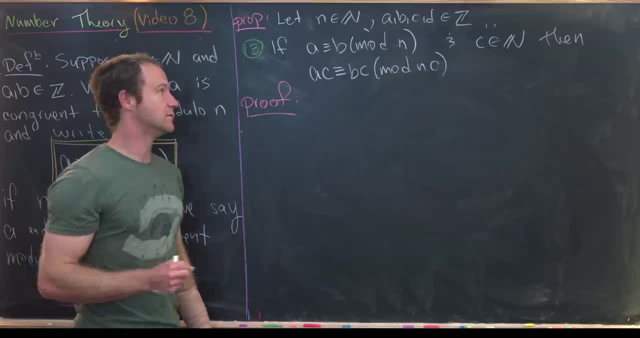 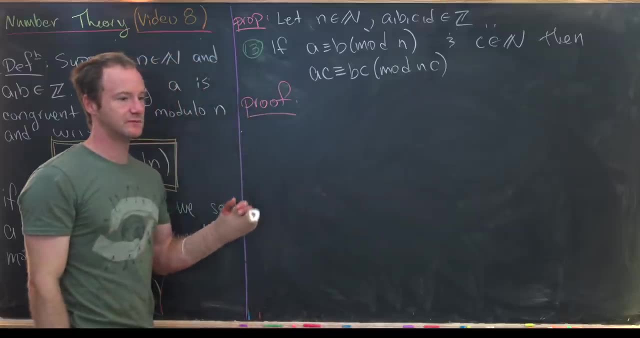 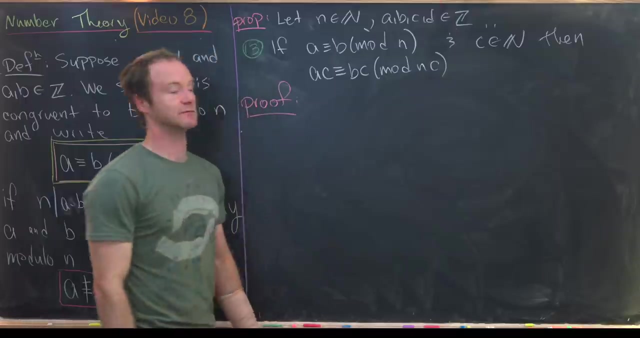 converse, but it sort of looks like one, because we are building up what we are, reducing modulo. So before we went from reducing modulo n to reducing modulo a divisor of n, And here we're going from reducing mod n to reducing modulo a multiple of n. Okay, so let's maybe get to it. 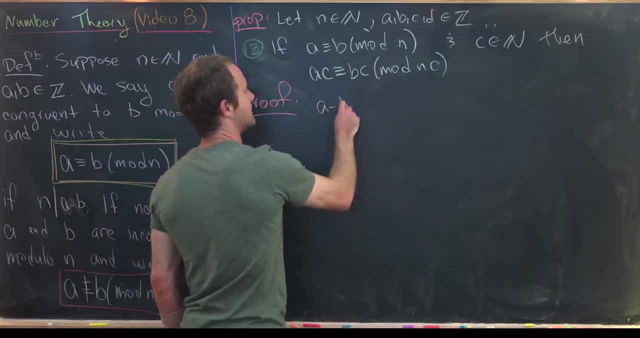 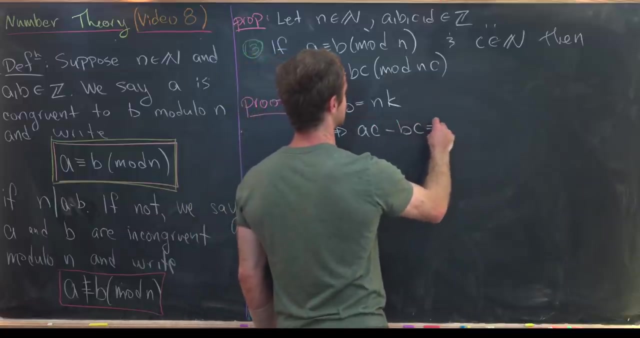 So let's notice that this statement right here means that a minus b is equal to n times k. And now this is actually really quick. All we have to do from here is multiply this entire equation by c, So that'll give us: ac minus bc is equal to nc times k. 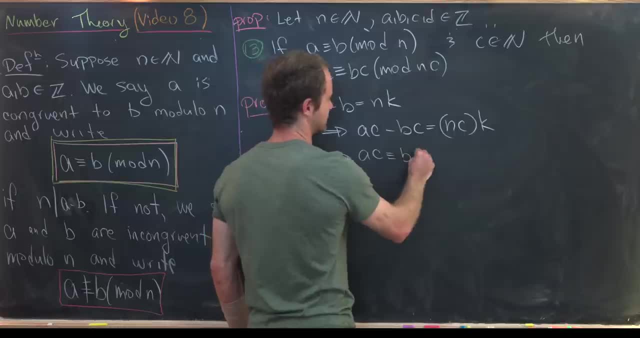 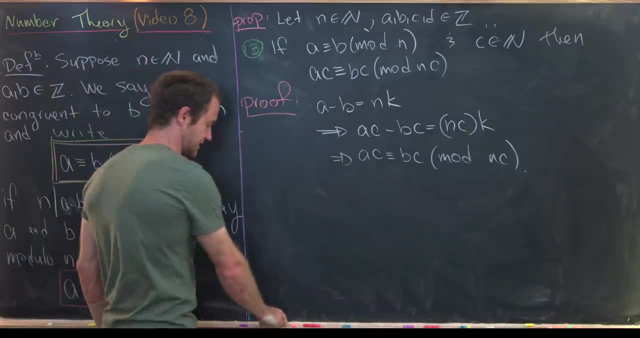 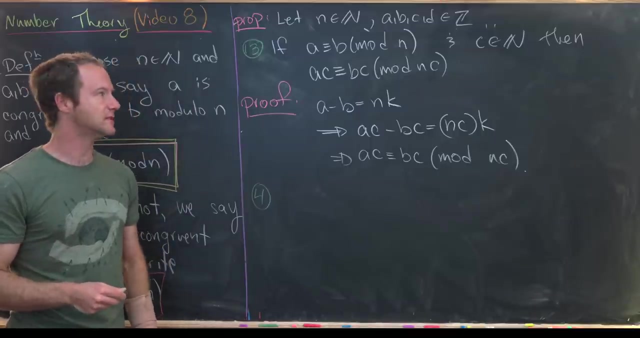 Exactly what it takes for ac to be congruent to bc modulo nc. Now I said there was a fourth part of this proposition, but I'll either leave the proof for you or just notice that it will immediately follow from what we did in the first part. 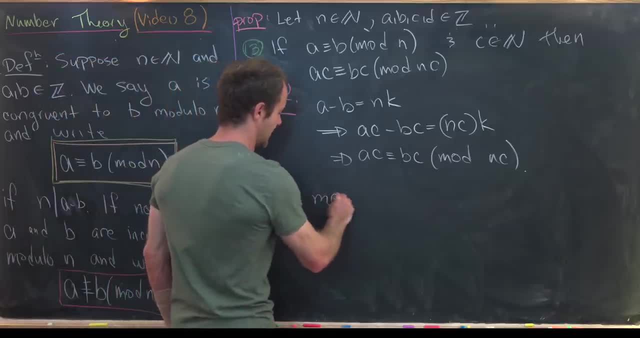 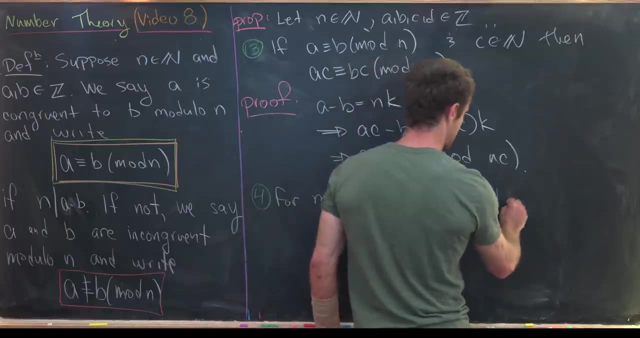 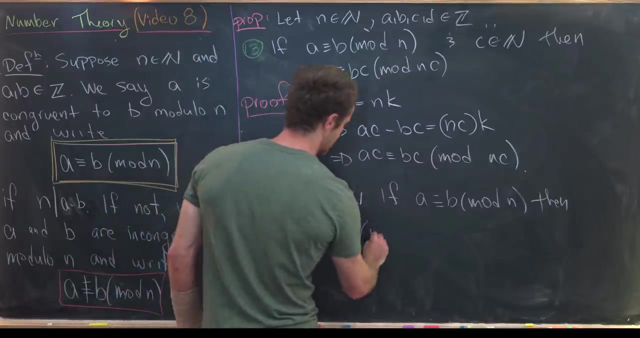 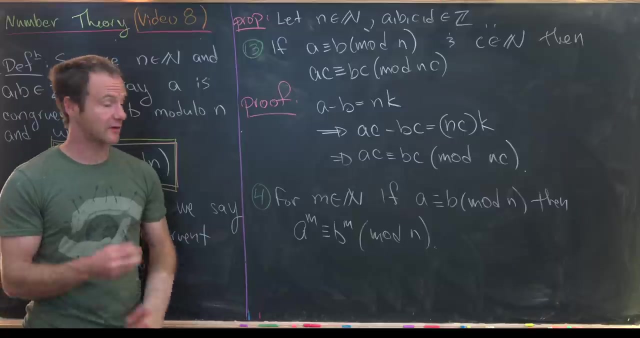 And that goes like this. So for a natural number, m, if a is congruent to b mod, then a to the m is congruent to b to the m modulo n. Okay, good. So now that we've taken care of this arithmetic proposition, we're going to look at. 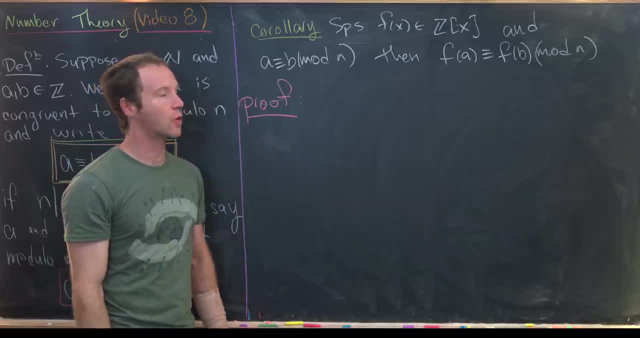 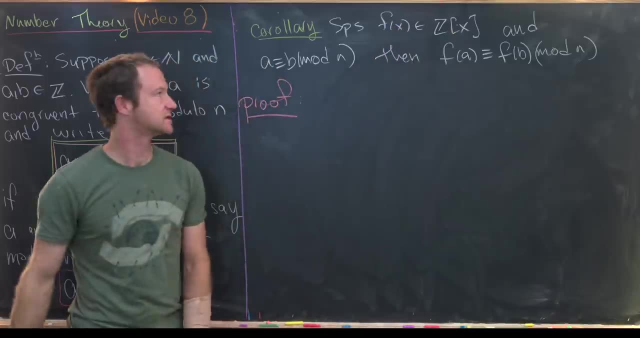 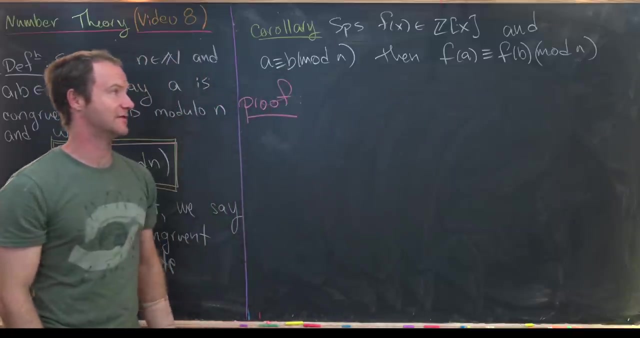 some results that follow from it. We'll finish with a quick corollary which follows from that last proposition. So if we've got a polynomial with integer coefficients and we know that a is congruent to b mod n, then f of a is congruent to f of b mod n. 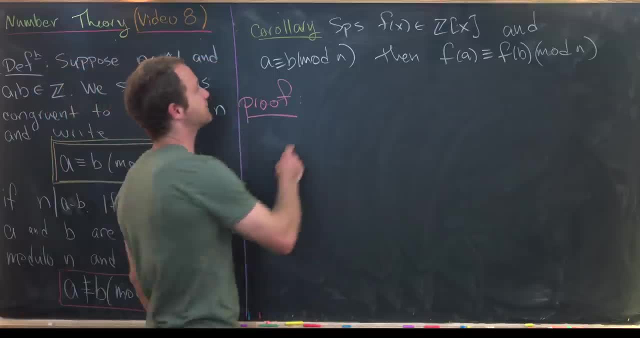 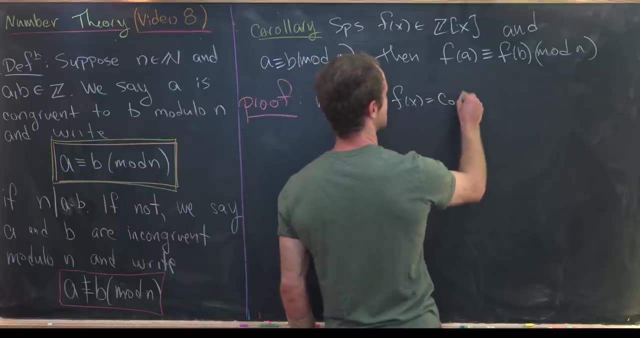 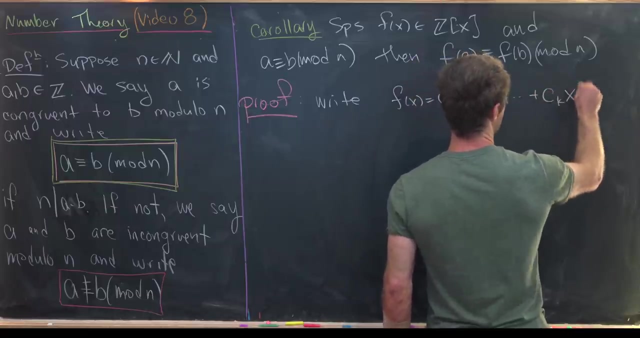 So this proof is actually quite short, but we're going to look at it anyway. So let's maybe write the polynomial as follows: We'll say f of x is equal to c0 plus c1 times x plus all the way up to ckx, to the k. So it's going to be a degree k polynomial.